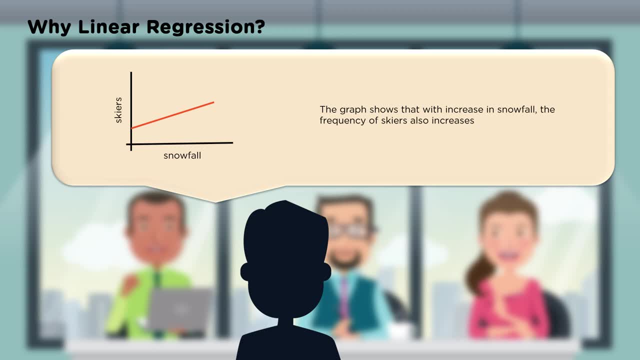 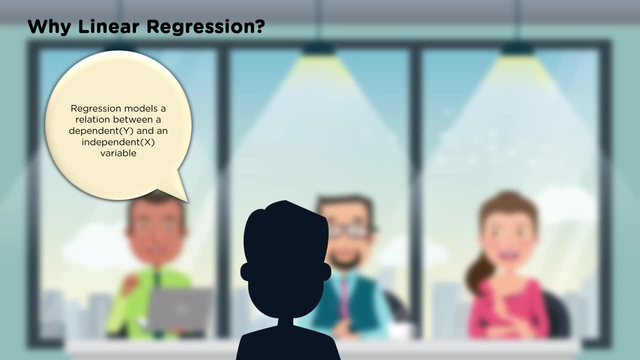 Thus we see that the number of skiers are directly proportional to the amount of snowfall. Regression models, Regression models, Regression models. And so it's interesting to see the difference between a dependent Y and an independent X variable. And so it's interesting to see the difference between a dependent Y and an independent X variable. 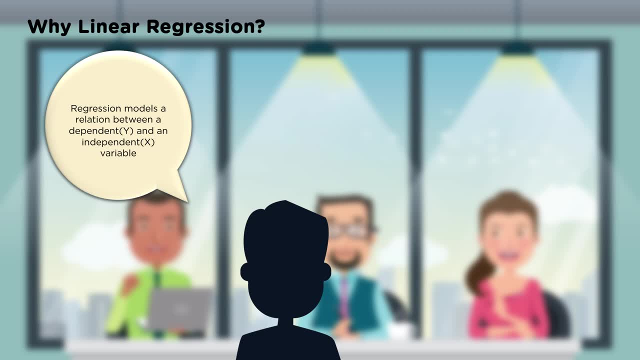 This is real important to understand regression, because we talk about linear regression. it's the basis of almost all our machine learning algorithms out there And it's usually an underlying part of the math in our deep learning. So it all starts here with linear regression. 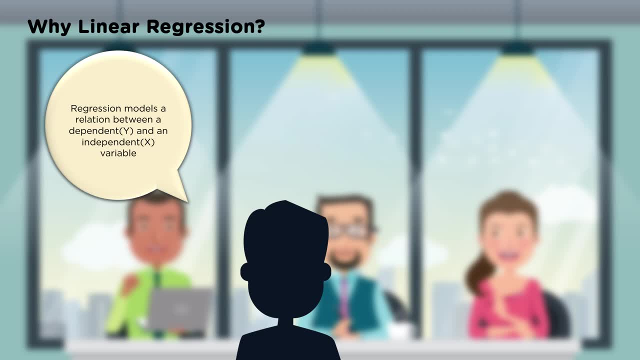 And we talk about a dependent Y and an independent X variable. these are numbers. We're usually talking about floats. We're usually talking about floats categorical, where we want to know yes or no, true, false. So regression means we're looking. 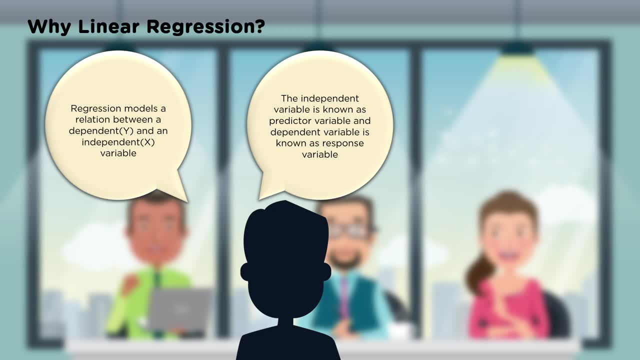 for a number. The independent variable is known as predictor variable, and dependent variable is known as the response variable. So we have one predictor variable- the amount of snowfall- and one response variable- how many skiers are going to show up- And then we can take this: 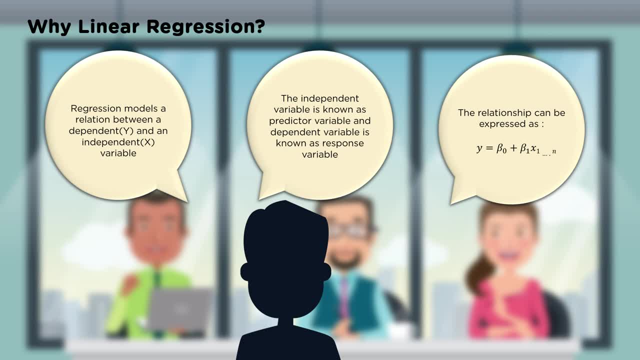 relationship and it can be expressed as: y equals beta. We're going to use the Greek letter beta and we have beta naught plus beta 1, x1, and if you continue out, it'd be plus beta 2, x2,. 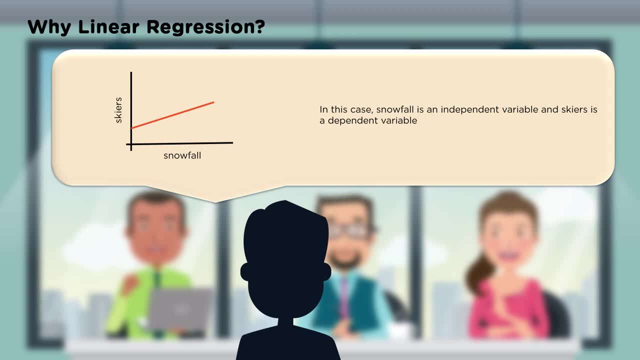 and so on until the nth degree. In this case, snowfall is an independent variable and skiers is a dependent variable. So we kind of had a little quick overview. Let's go ahead and talk a little bit more about what is linear regression. So we're going to go from y predicting a number. 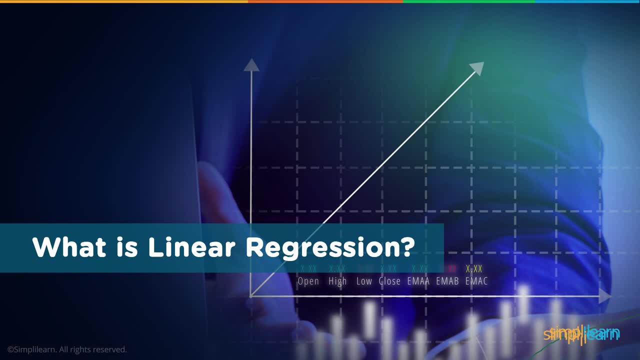 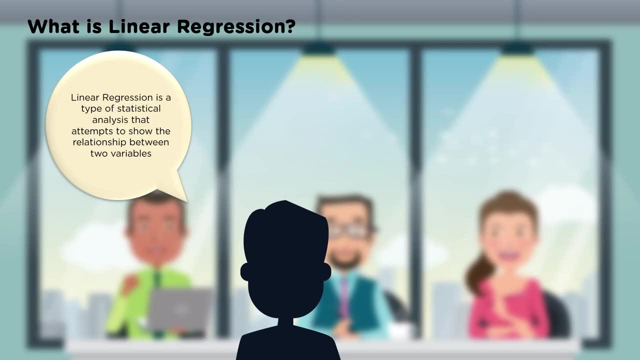 of skiers for snowfall, and we've looked at the formula a little bit. but let's look a little bit closer at what exactly is going on with linear regression. And the question is going to come up in an interview: What is linear regression? Linear regression is a type of statistical analysis that attempts to 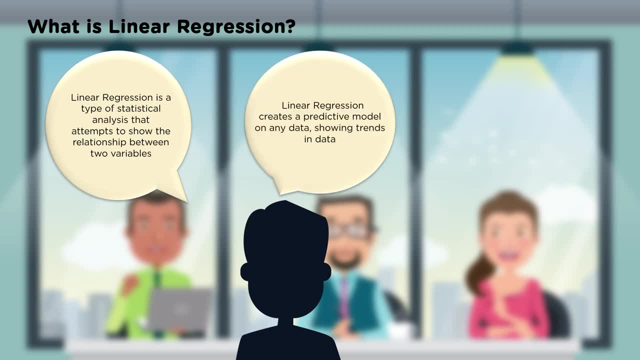 show the relationship between two variables. Linear regression creates a predictive model on any data showing trends in data. The model is found by using the least square method. There are other methods. The least square method happens to be the most commonly used out there. 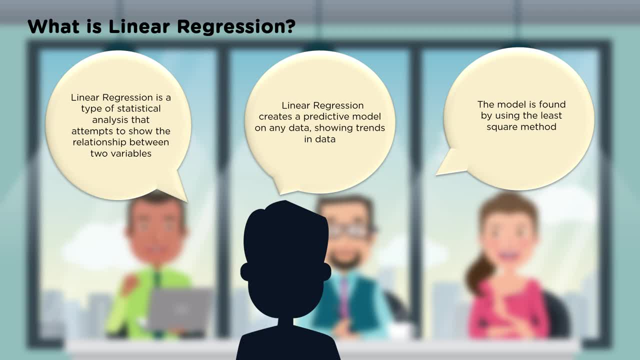 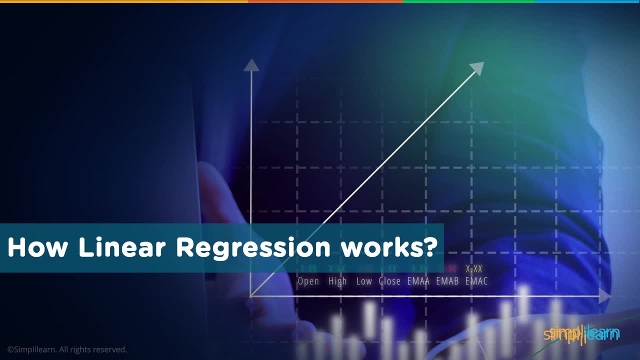 and we usually start with the least square method, since it's the most common and usually works the best on most models. And we're already looking at how linear regression works, but let's dig deeper into it and let's take a closer look How linear regression works. I will 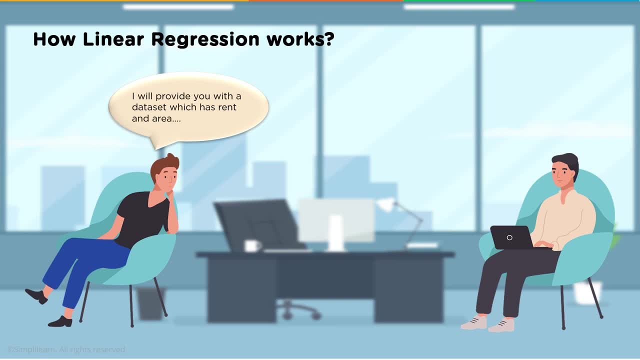 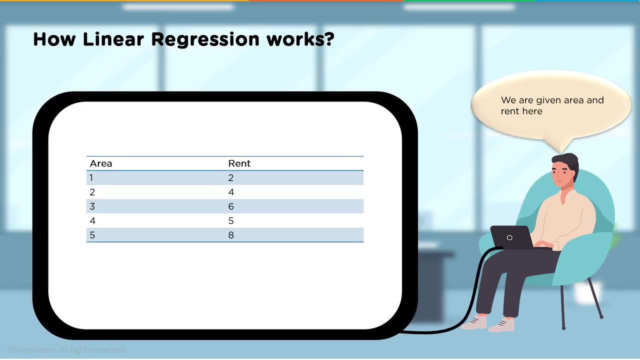 provide you with a data set which has rent, area, other information in it. It looks like our secret agents have put on their casual wear for this one. You need to predict rent accordingly. We are given area and rent here, So you can do linear regression with more variables. but we're just going to look. 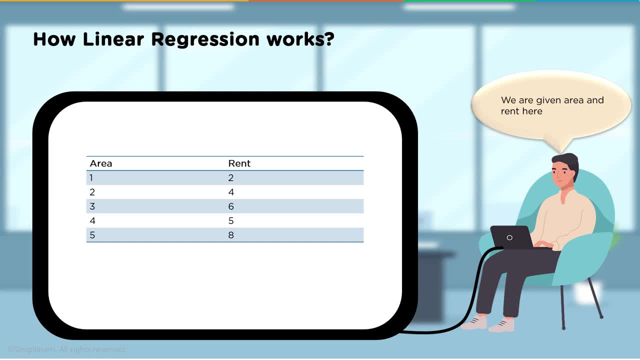 at the area and then from that try to figure out what the rent should be. We plot the graph and if you look at it here you can see that the graph is kind of a little bit different. It's a linear pattern with a little dip in it. So the area seems, the rent seems to be based on. 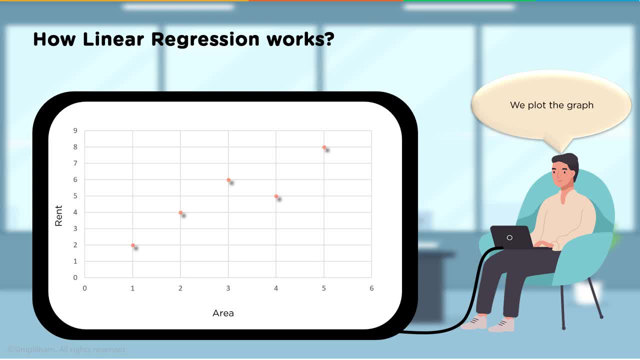 the area. In most of our work as data scientists, we usually try to start with a physical graph, if we can, So we can actually look at it and say, hey, does what I'm fitting to this graph look right? You can solve a lot of problems that arise by looking at the graph and saying no. 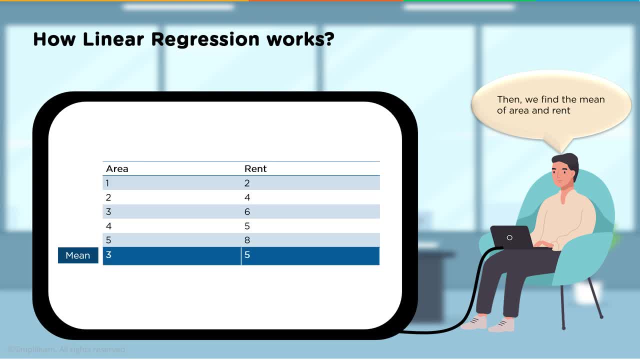 that doesn't look right at all, Or oh, I should be looking over here for this. Then we find the mean of area and rent. So the mean just means average. And if you take a look at the graph, take one, two, three, four, five and add them all together and divide by. in this case there's. 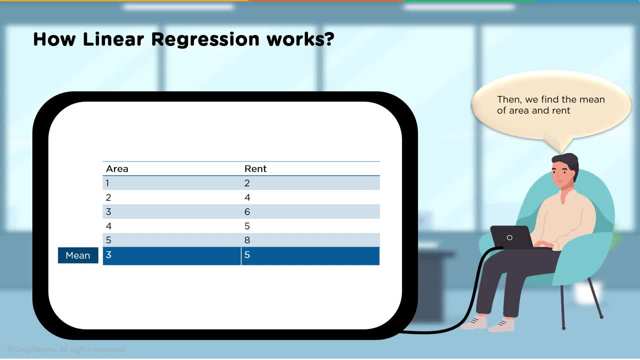 five areas, you get three, And the rent is two, four, six, five and eight. If you add them all together and divide by five, you get five, And we plot the mean on the graph So you can see right. 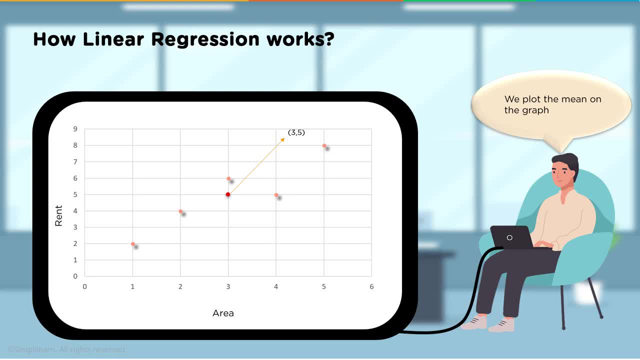 here. here's the mean of the rent and the area. It's kind of a very central point, which is what we're looking for. the average of everything in there, The best fit line, passes through the mean. This is real important When you're eyeballing it. as humans, we can do this fairly easy. if it's a 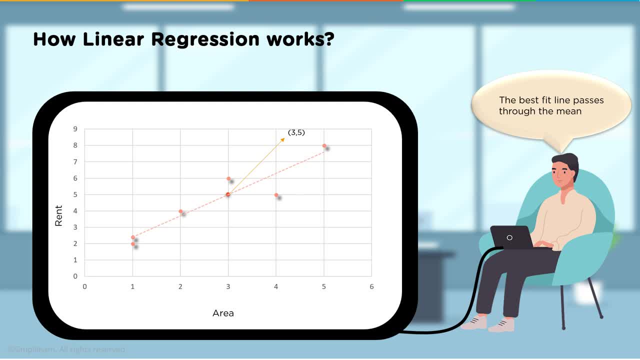 straight line through a bunch of data. It gets more complicated mathematically when you start adding multiple variables and instead of a line you have a curve. But for basic linear regression we're going to draw a line through the data And the line should go through the means. That's going to be part of the best fit for that. 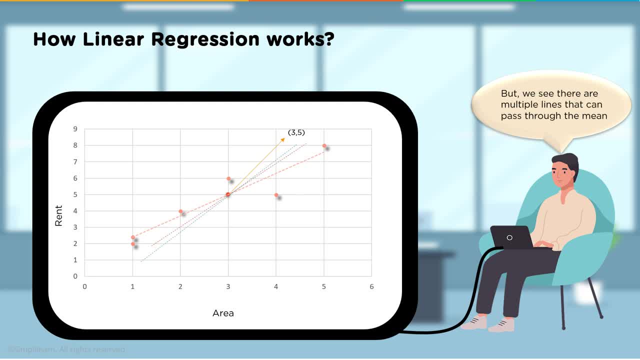 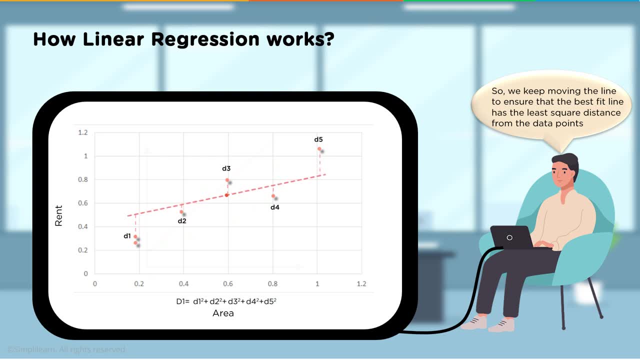 line. But we see there are multiple lines that can pass through the means. So, depending on how you look at it, you can kind of wiggle the line around back and forth. So we keep moving the line to ensure that the best fit line has the least square distance from the data points. And this is you. 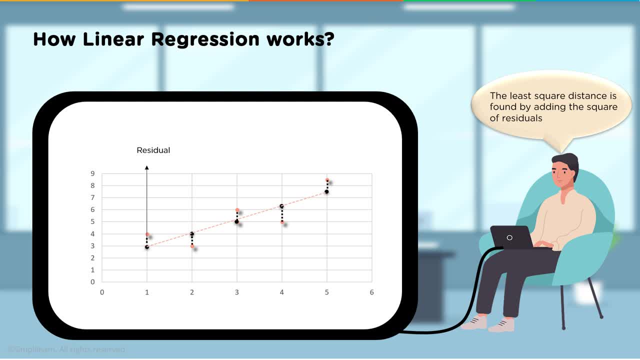 can see right here, residual. We have our data point and then we look at the distance between them and we square that distance, And that's what they mean by the least squared distance. We want all those distances to add up to the smallest amount. we 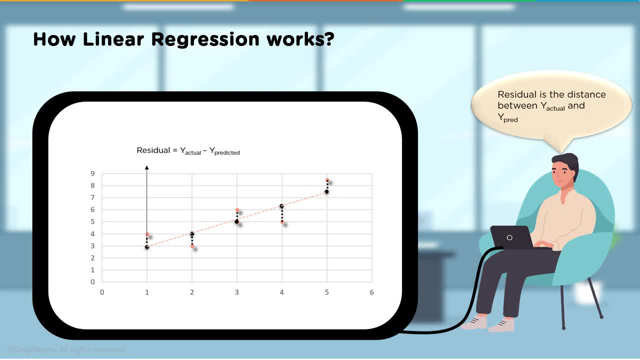 can. When we talk about that distance, we call it the residual. It equals the y actual minus the y predicted. Very straightforward: We're just looking at the distance. You can accidentally switch these and it will come out the same because we're going to square it. But when you're working with other sets of linear regression. 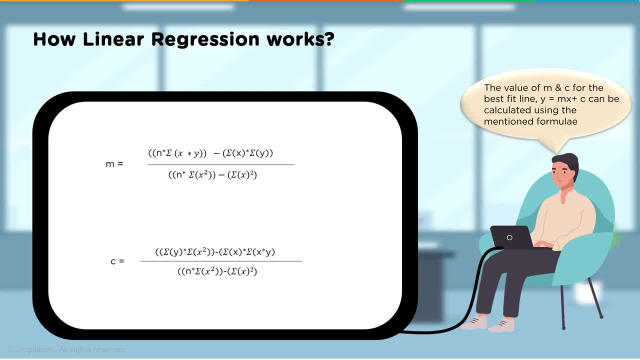 you want to make sure you do the y actual minus the y predicted. The value of m and c for the best fit line, y equals mx plus c can be calculated using the mentioned formula And you can see here we have: m equals the number of. 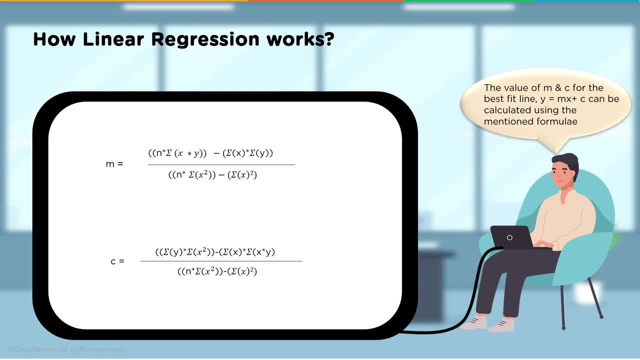 points. that's what n stands for. Then we have the sigma. the Greek symbol is there, which is a summation of x times y minus the summation of x times the summation of y over the number of the summation of x squared minus the. 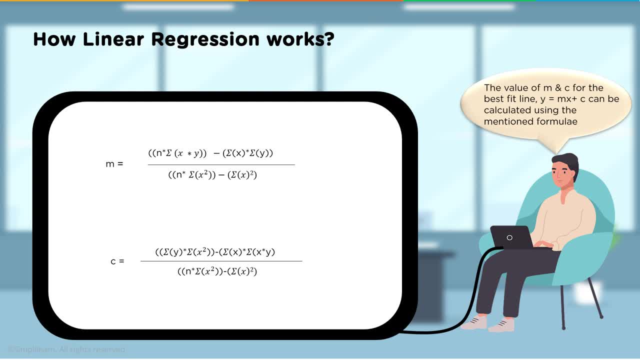 summation of x squared of x all of it squared. That can be a little confusing trying to say that. And then, of course, your c value is going be the summation of y times the summation of x squared minus the summation of x times the summation of x times y over the total count of the. 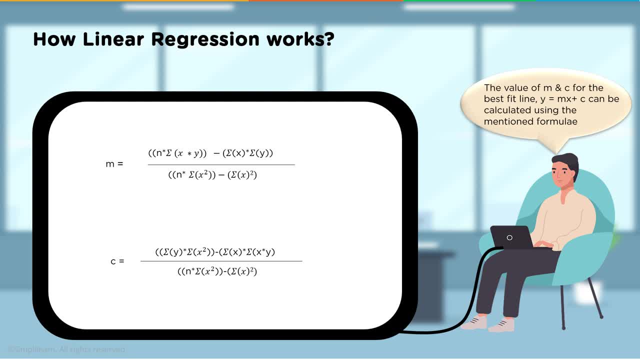 summation x squared minus the summation of x squared. That's a mouthful. Normally we don't worry too much about these formulas, other than to know they're there. Now, if you're a mathematician, you might go back in there and work on those. 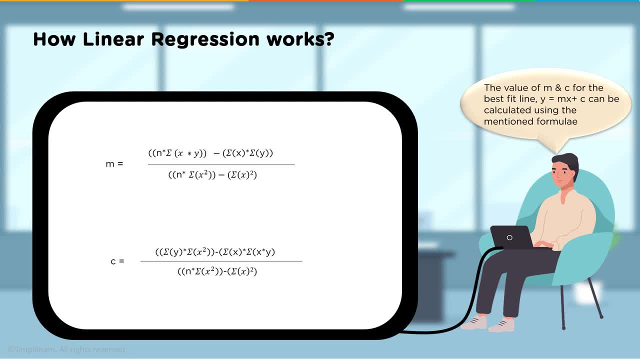 and those people who originally started to put together the different models in R of course had to know all this math to build them and had to test it out. That's one of the nice things about R. What is important is that you know about these. 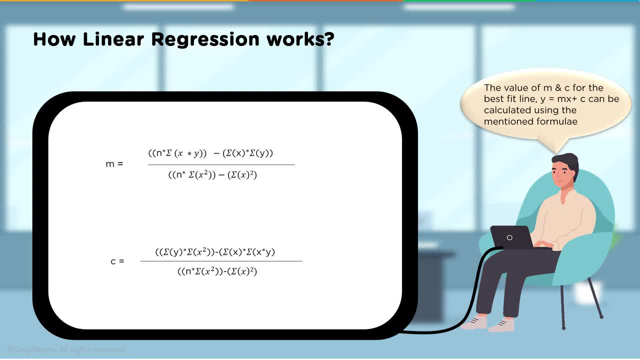 formulas so that you know where it's coming from. So if you're using one linear regression model, this is how this one works. There's other linear regression models based on different math, and so you'd have to be aware when that math changes and how that changes the model. We find the corresponding values, So in 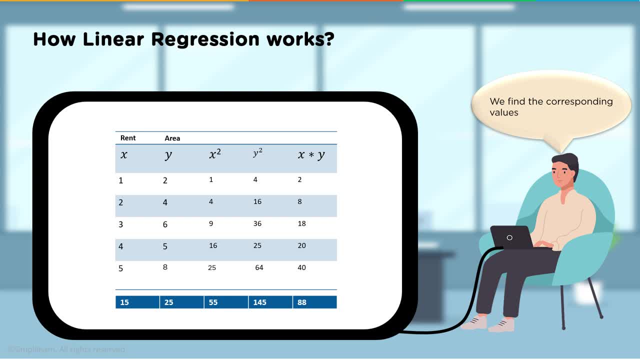 this case, if you're going to break this up and you're building your own model instead of using the one in R, you would have your rent, you would have your area, you would find your rent squared, your area squared and your rent squared. 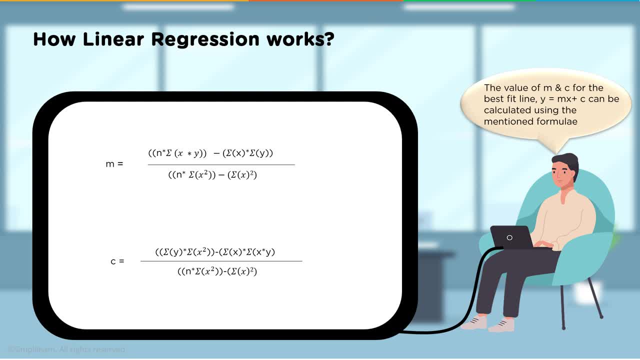 times area And if we go back one, we can see that that's all the different little pieces in this model. We have x times y, we have x squared, we have the sum of x which is going to be squared, we have the sum of x, the sum of y. This is the same. 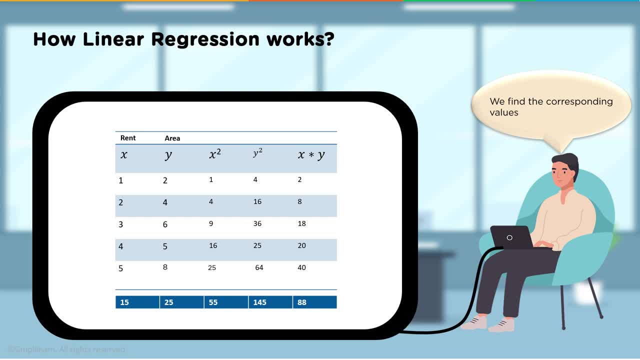 These are all the little pieces in here that we see for m equals and c equals, And so once we compute all these, we have 15,, 25,, 55,, 145,, 88.. Very easy to do on a computer, thankfully. You could have millions of these points and it would do. 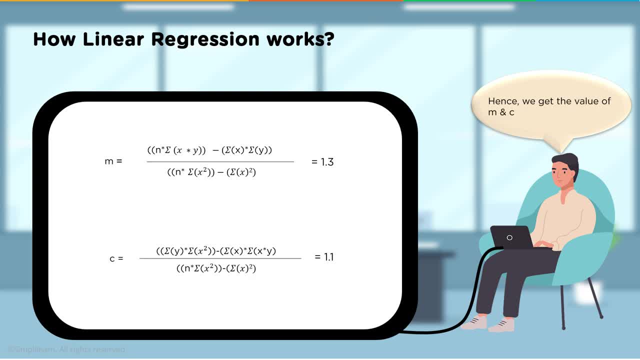 it in a very short period. Let's plug in those values very easily into this formula and get a final answer, And we'll see that m equals 1.3 and c equals 1.1.. And then when we take this for the y predicted equals m of i, x of i plus c. we can take these and actually 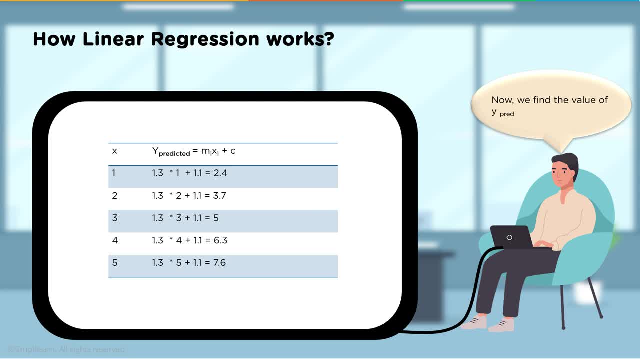 run the data we have. So we're going to see how it predicts. So now we find the value of y predicted, So we have our x in and we want to know what we think y will be based on our formula. we generated the linear regression formula. 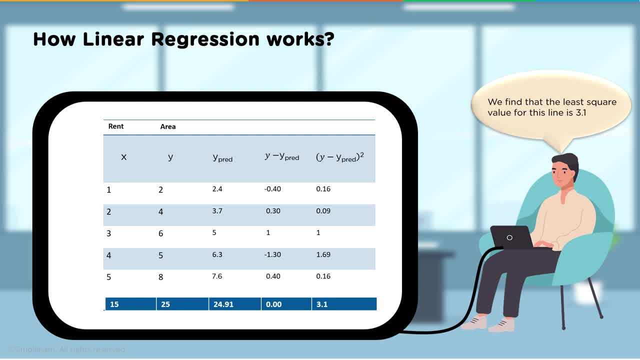 And so when we come in here, we have our x, we have our actual y, then we have our y predict what we think it's going to be. And then we have: we take y minus y- predict and we get those values minus 0.4, it's off by 0.3, this one's off by 1,. 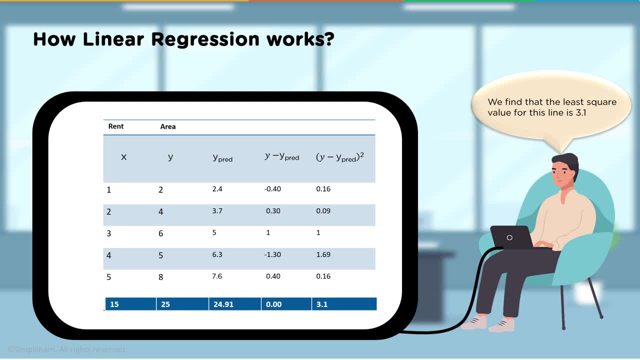 this one's off by minus 1.3,, by 0.4.. And we go ahead and square that and then we can sum that square and average it out and we'll get a value. This is just a summation down here of y minus y. predicted square is 3.1.. 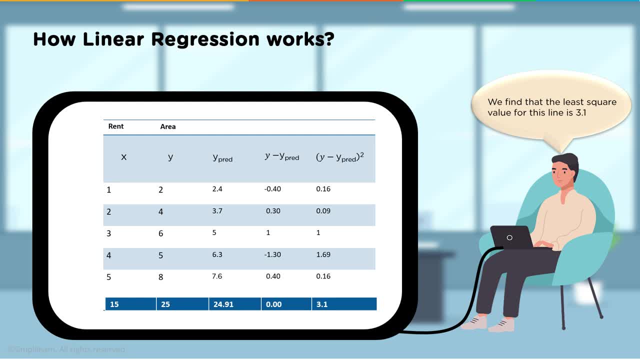 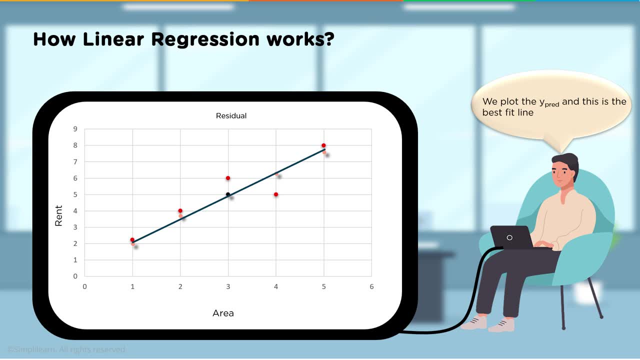 And we call that. the least square value for this line is 3.1. And we go ahead and divide that by 5.. So when we plot the y predict and this is the best fit line, and you can see that it does a pretty good job going right through the middle. 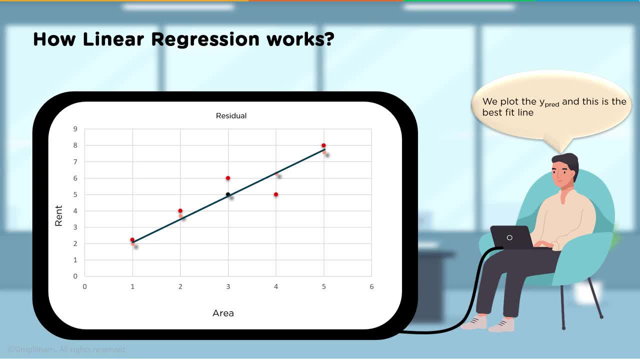 of lines And in something like rent versus area. if you're trying to figure out how much rent to charge or how many people are allowed to be in the area, that's going to work. But if you're looking for the rent value compared to, 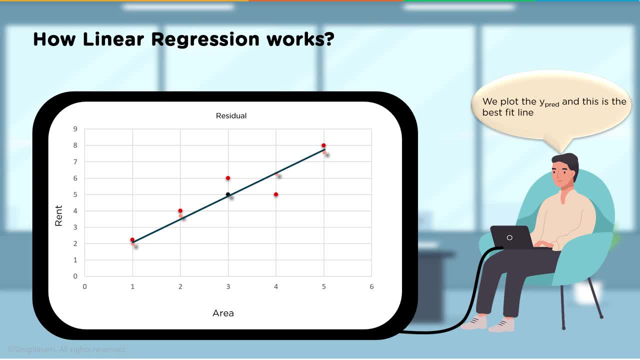 the area. this gives you a good idea, based on the area, of what you should rent the place for. It's close enough that in the business world this would work. You're not computing something down to the millimeters or micrometers or nuclear physics. We're just charging people And 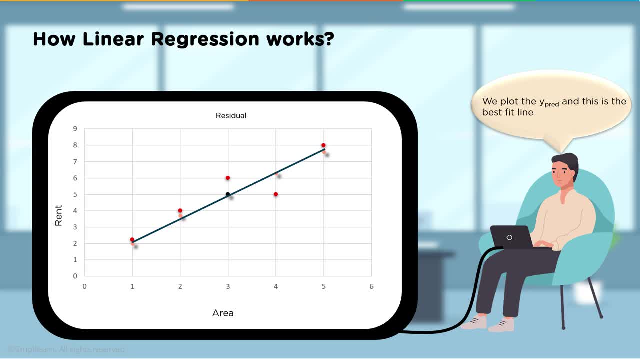 so if you're off by a couple dollars it's not a big deal. You'll be pretty close to what you think it's worth and get the right value for your property. Use case: Predicting the revenue using linear regression. Now that you have a, 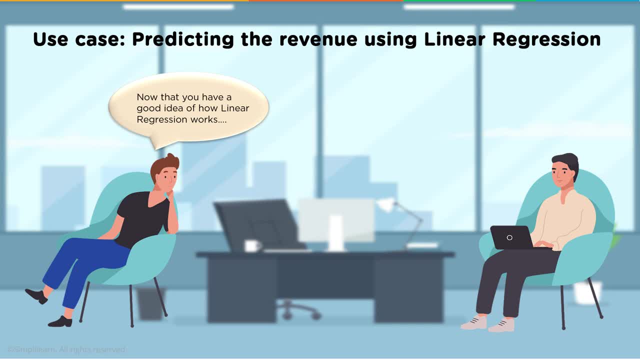 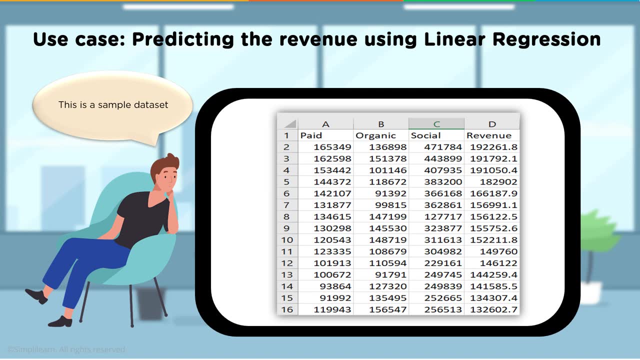 good idea of how linear regression works and we're kicking back on our lounging sofa today. let's work on a real-life scenario where you have to predict the revenue. So we're going to take a data set and we'll pull this up in just 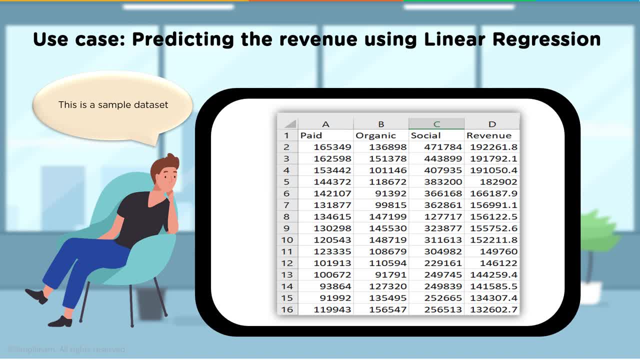 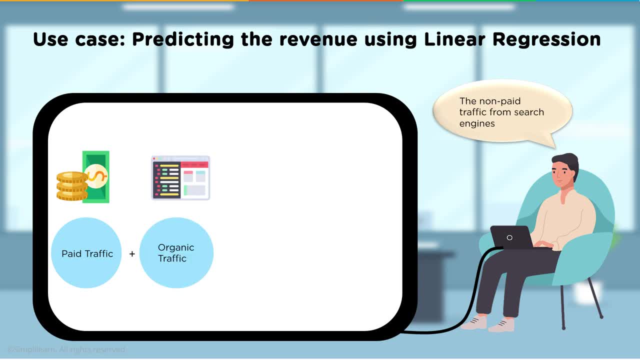 a minute We'll have paid organic, social and revenue. There are three attributes we'll be working on. The first one is our paid traffic, So all the traffic through the advertisement that comes in The non-paid traffic from search engines. So 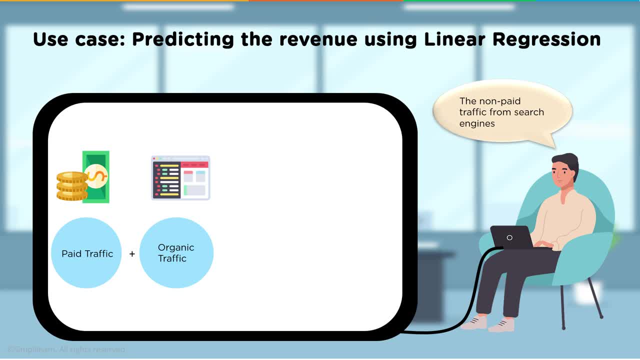 these are people coming to the website and are doing so because they did a search for something specific, So it's pulling it from your website- All the traffic coming from social networking sites- So we want to know what's coming from Twitter and Facebook and somehow they've linked into your website and 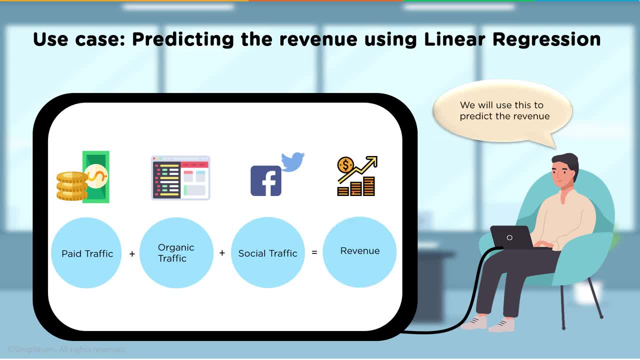 coming into your marketing area to buy something, And we'll use this to predict the revenue. So we want to know how all this traffic comes together and how it's going to affect our sales. if the traffic is coming in, We're going to make use of the multiple linear regression model. So 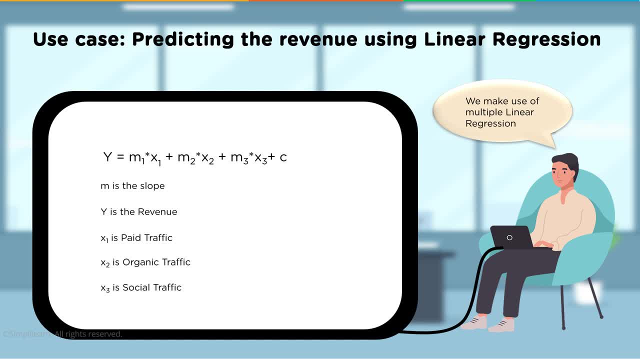 you'll see that this is very similar to we had before, where we had y equals m times x plus c, But instead we have y equals m1, x1 plus m2, x2 plus m3, x3 plus c. M is the slope, So you have m1, m2, m3.. The three different slopes of three. 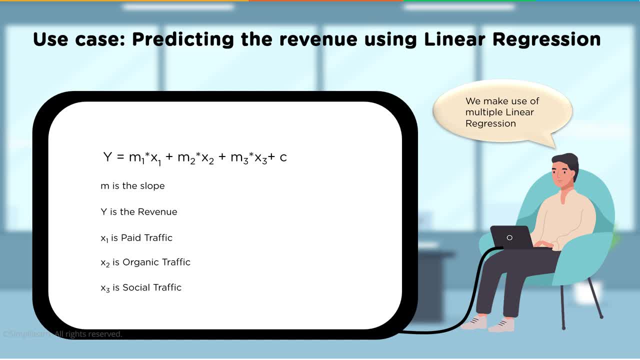 different lines. Y is the revenue, So we're only looking for one variable And remember, this is regression. so we're looking for a number. X1 is going to be the paid traffic and, of course, m1 the corresponding slope, X2 the organic traffic and x3 the social traffic. We 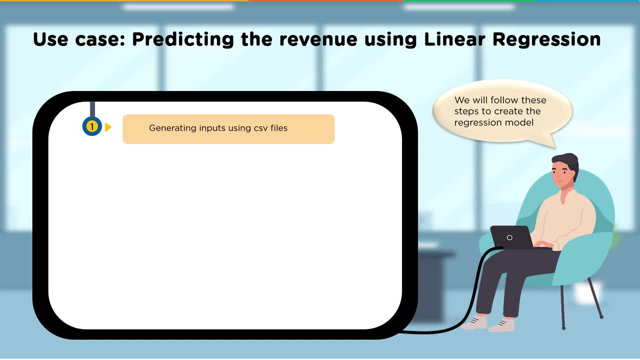 will follow these steps to create the regression model. We'll start by generating inputs using the CSV files. We'll then import the libraries, Splitting the data into train and test- Very important whenever you're doing any kind of data science: Applying regression on paid traffic, organic traffic, social. 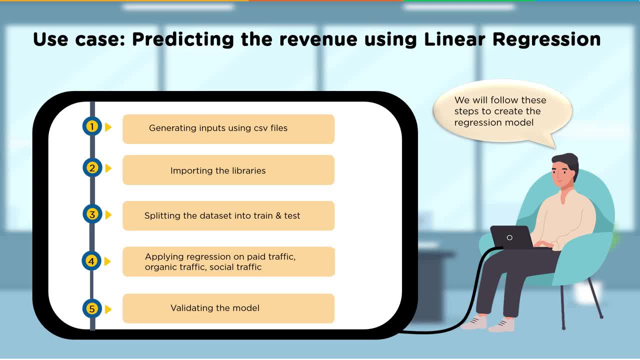 traffic. So we're going to apply a regression model on them And then we're going to validate the model. That's the whole reason we split it to a. training and testing is so we can now validate to see just how good our model is. 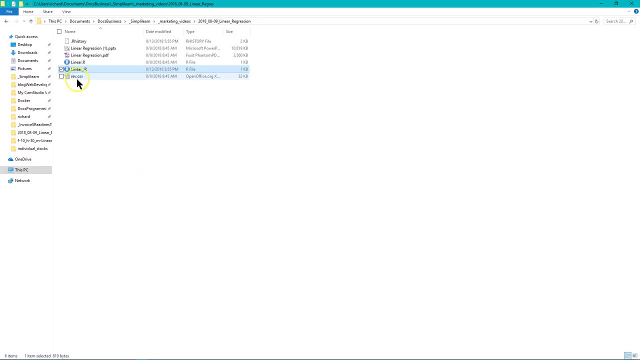 Now, before we open up R, I always like to just take a quick look at the data itself. And we're using the revcsv file And this is a cs file or a comma separated variable file. We'll just open that with WordPad- Any kind of text. 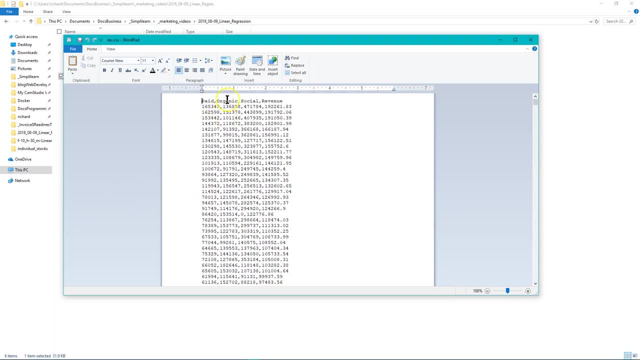 editor would be nice to show you what's going on And you can see. we have paid organic social and revenue across the top. This is your titles for your columns And the value is going down And this is the same as what we saw on the slide just a minute ago: Paid organic social and then 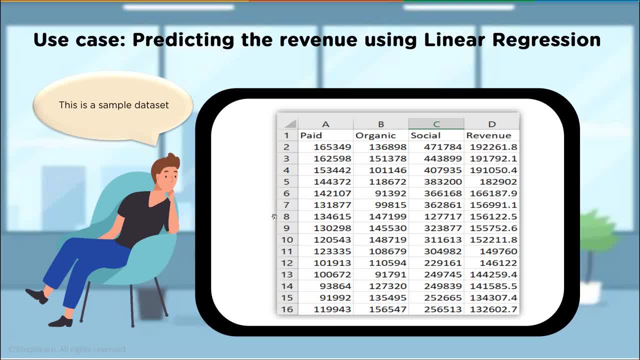 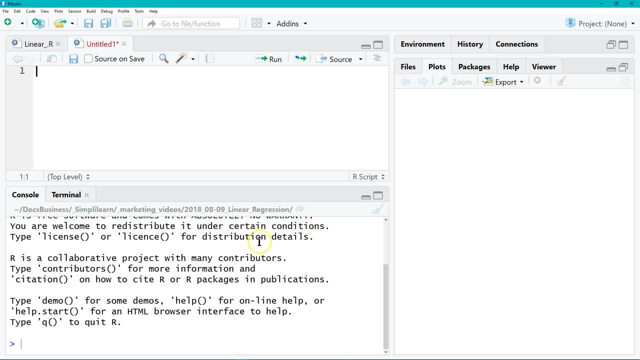 revenue from them. They probably have it in more of a spreadsheet than just a WordPad And I'm using the newer version of RStudio, which already has a nice layout. It automatically opens up with your console terminal window. down and left You have your script And we'll run it in script And then, when I run it, line: 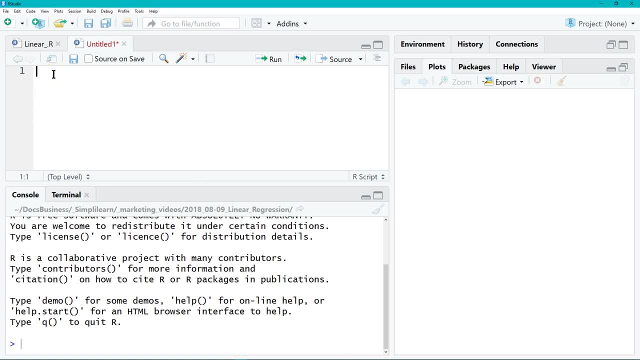 by line in script. you'll see it show up on the console bottom left. I could type it straight into the console and then run it line by line in script. You'll see it show up on the console bottom left. I could type it straight into the console. 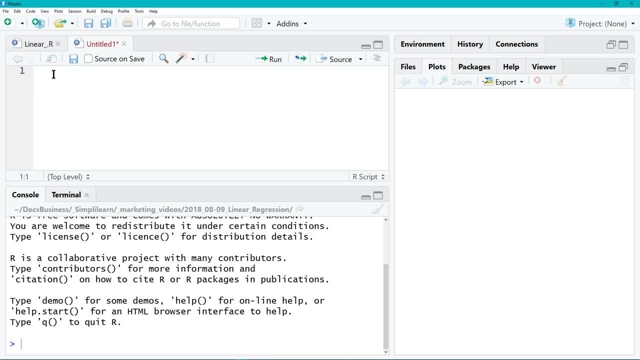 and it would do the same thing. And then on the right, we have our environment, And under the environment we'll see plots. If you're in an older version, the plots will pop up And you usually are running just in the console, And then you 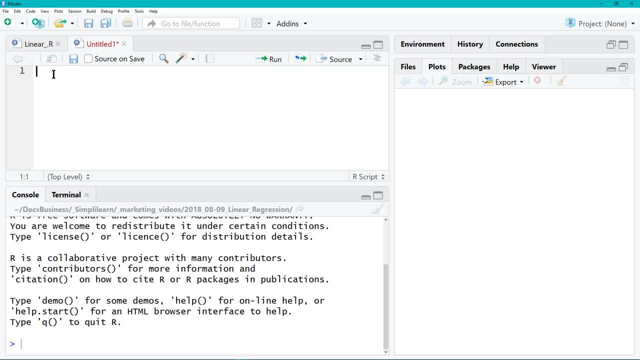 have to open up a different window to run the script, And you can run the script from there. This opens up everything at the same time when you use the new RStudio setup, And the first thing we want to do is we want to go. 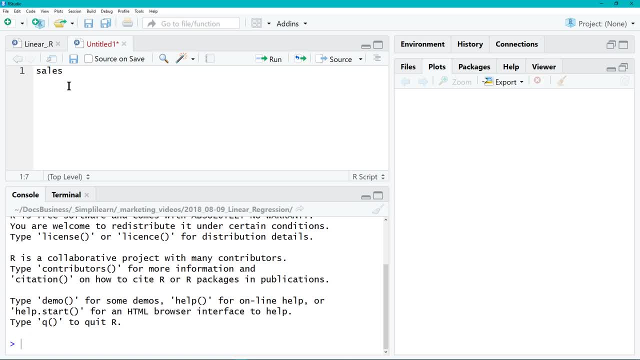 ahead and generate a variable. We'll call it cells, And we want to load this with our data set, And so in R we use the less than minus sign. That's the same as assigned to. It's like an arrow pointing at cells. 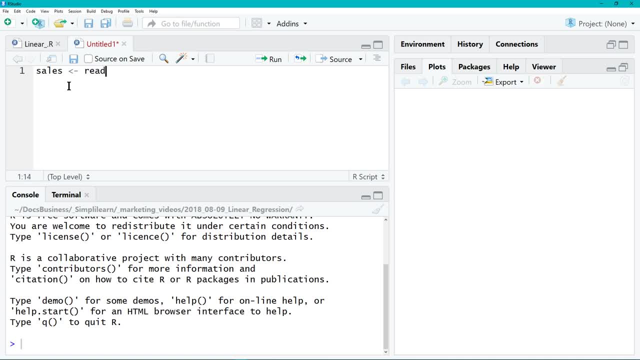 And it says: whatever it goes past here is going to be assigned to cells And we want to read in our CSV file. And then I went ahead and fixed the CSV file up a little bit. When I say the CSV file, I mean the path to it. We'll go ahead and just paste that in. 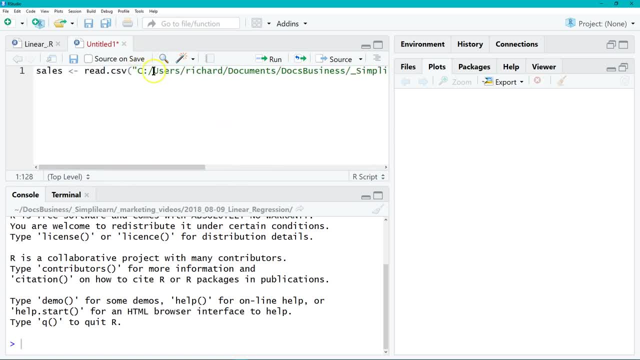 there And this is my edited version And you'll see I took wherever we had the backward slash, I switched it for a forward slash, Because a backward slash is an escape character And when you do that, you're going to see that the 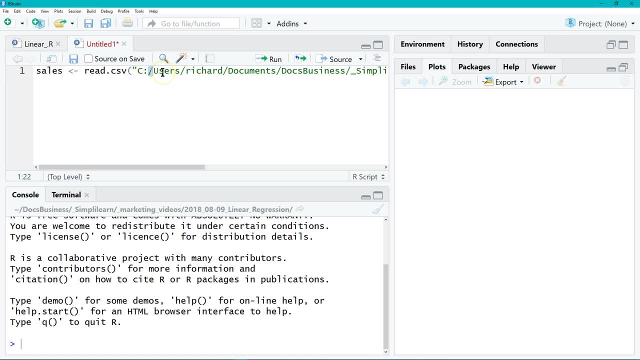 path is going to be assigned to cells. So whenever you're programming in just about any scripting language, you want to do the forward slash instead. So, like a good chef, I prepped this and copied it into my clipboard And we can see the 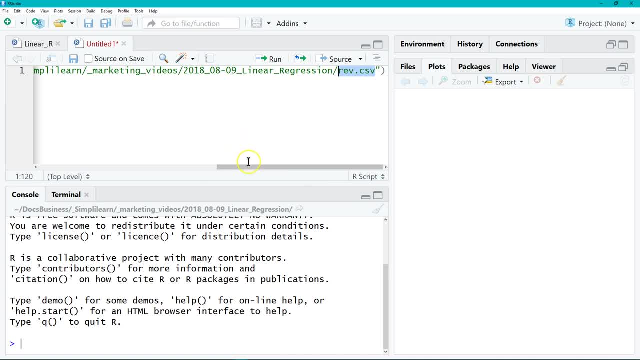 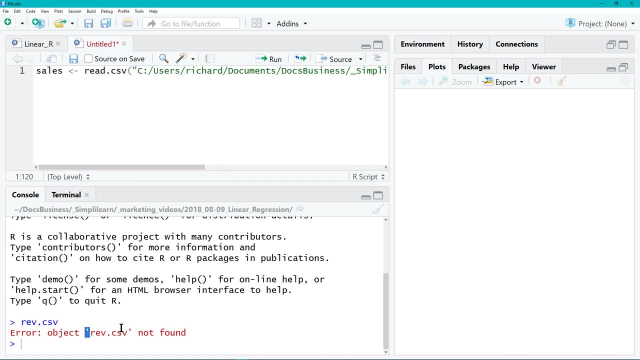 full path here And the full path ends in our revcsv file. So that's the path on my machine And then I'm going to run that And now we have down here. you see it appear right here. Uh-oh, it must have an error in my path. It says object: rev not 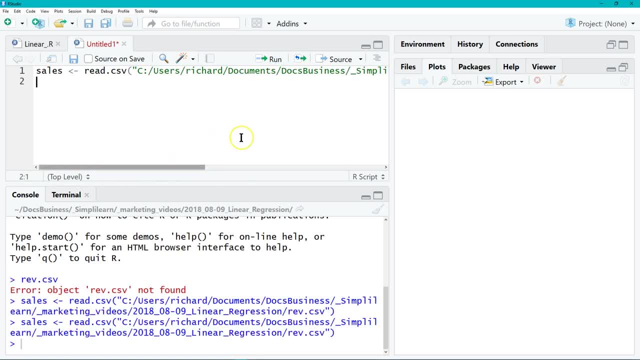 found. Let me fix that real quick And run it again, And this time it does assign the data set And then we'll just type in cells, And this is the same as printing it. So if you work in other languages you'll do like print and then cells, or 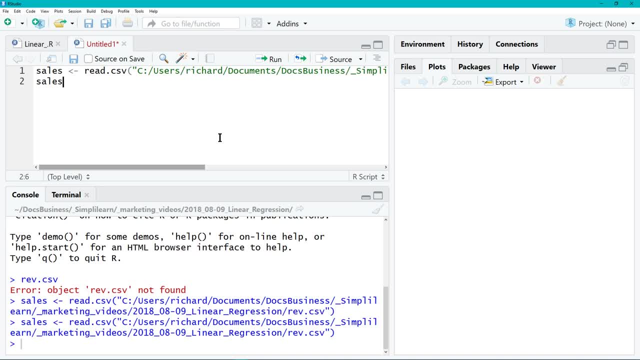 maybe print cells, dot head, if you're in pandas in Python or something like that, But in R you just type in the variable, We'll run this And you can see it printed out, all those columns. So that's the same thing we just looked at And it. 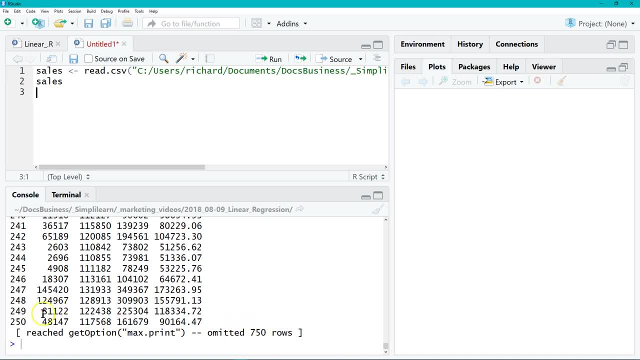 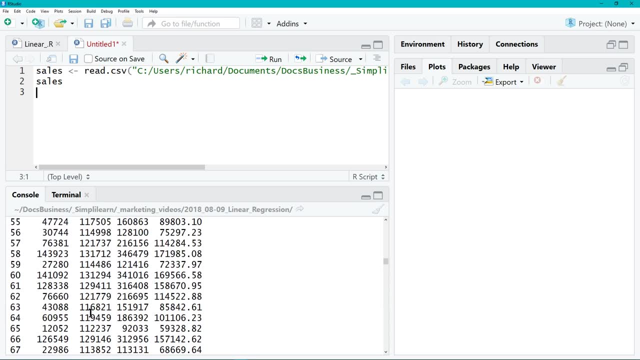 says max print, So it omitted 750 rows, So it has a total of 1,000 rows And we can scroll up here on our console where the answer came in. And if I scroll up to the top way up to the top, there we go. you'll see: paid, organic, social and 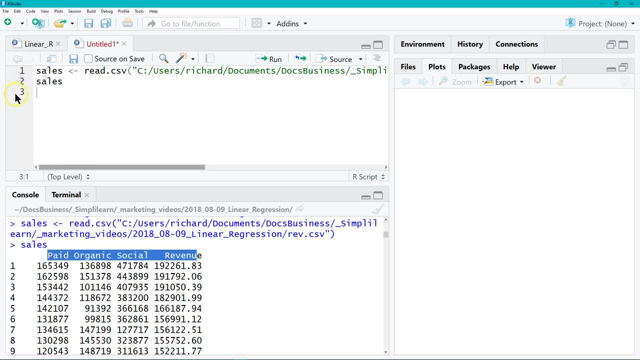 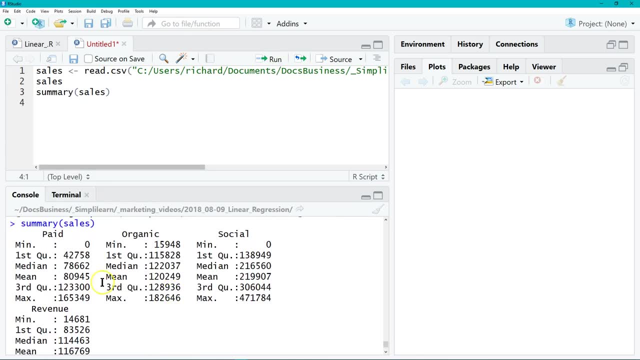 revenue. So everything looks good on this And there's a lot of cool things we can do with it. One of the things we can do is I can summary it. So let's do a summary of cells And we'll run that And the summary of cells comes in. It tells you: 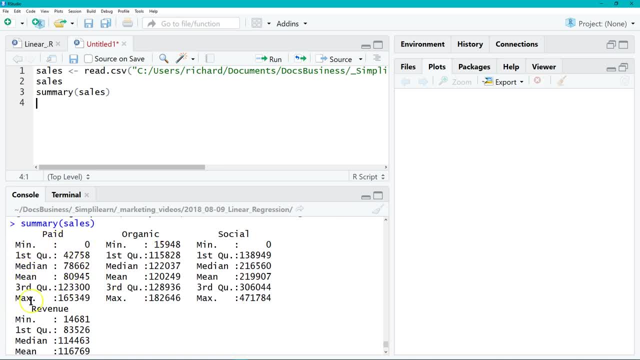 your min. first quarter median mean. third quarter max for paid organic social Breaks it up and you can actually get kind of a quick view as to what the data is doing. You can take more time to study this. A lot of people look at this. 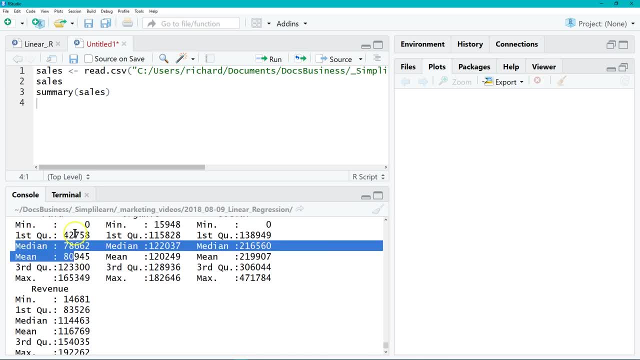 and it tells you a lot, And it's divided into quarters, So you have your first quarter value and your third quarter set up on there and max- It just gives you a quick idea of what's going on in the data. Summary is a really wonderful tool. 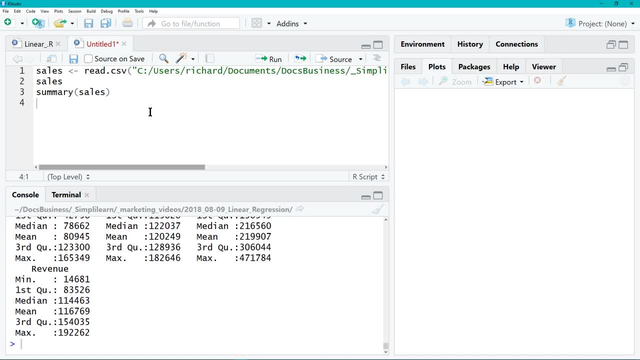 One of the reasons I like to jump into R before I might do a major project in something else. or you can run everything in R And let's take a look at the head, head of cells And let me run this And you can see. it just shows the head of our 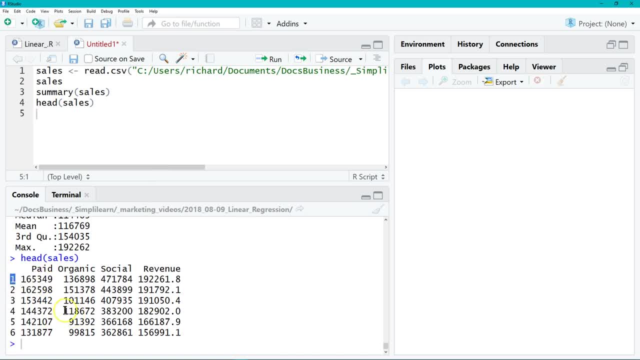 data, the first six rows in this case, And it starts with one Important to know. Systems start with zero and go up. R is one that starts with the first as one, And then, if we want to do a plot, I'll go ahead and do a plot. cells, Another, really. 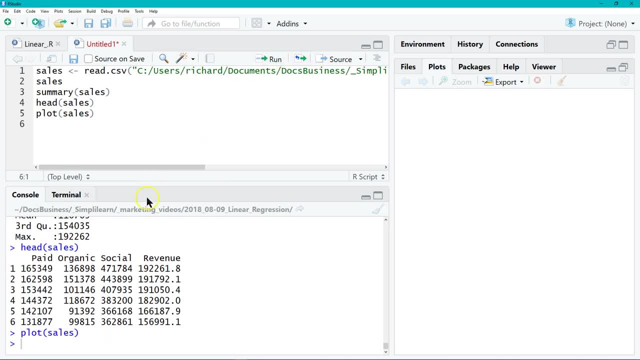 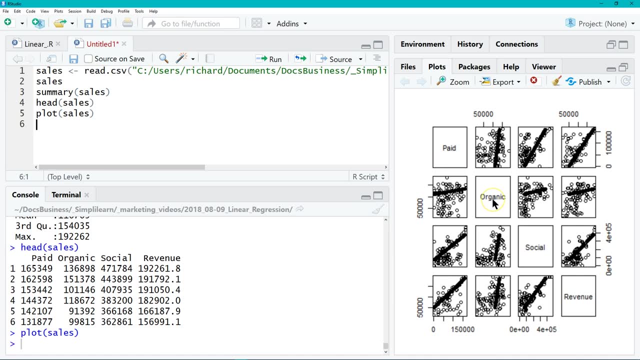 powerful tool that you can just jump right into with R once you have your data in here And you'll see that the plot comes over on the right-hand side, And what it does is it compares them. So if I look at my paid and my organic and you 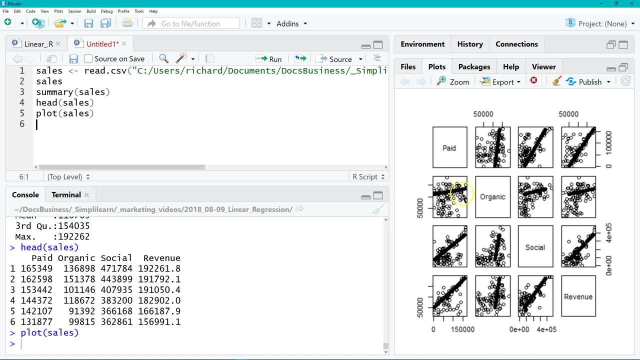 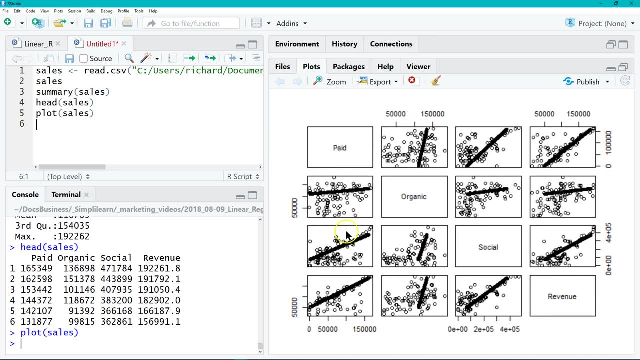 cross the two, you'll see there's a nice line down the middle big black line where it plots the two together. Let me just widen this a little bit so we can see more of it. There we go. Same thing with paid and social paid and revenue. So each one of these has a clear 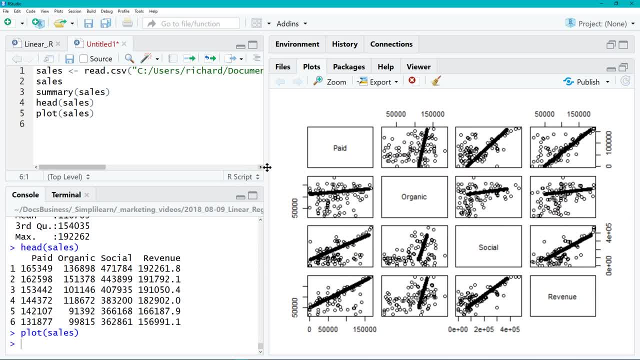 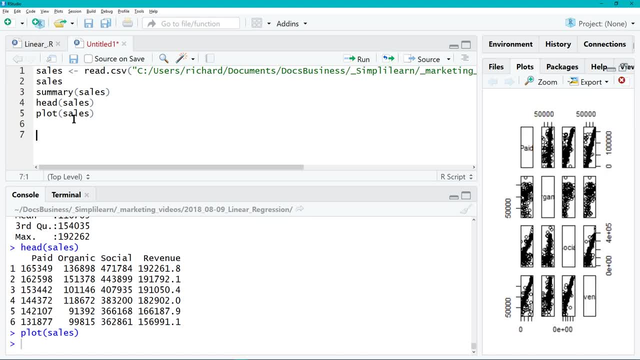 connection to each other. So that's a good sign. We have a nice correlation between the data and you can just eyeball that. That's a good way to jump in and explore your data rather quickly and see what's going on. So we'll go ahead and I'll put a pound sign there, a hashtag and splitting the data into 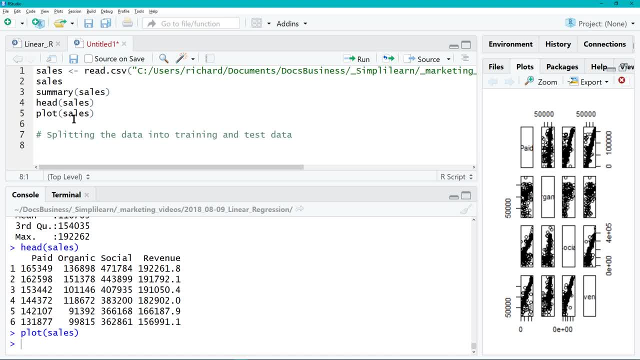 training and test data And we want to split it so that we have something to work with and train our data set. And when we do our data set, you do this with any data set because you want to make sure you have a good model And then, once we've trained it, we're going. 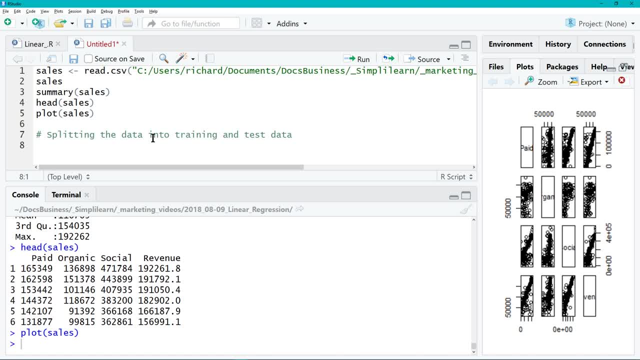 to take the other set of data we pulled off to the side and we'll test it to see how good it is. If you test it with the training data, it's already got that memorized and should give you a really good answer. In fact, when you get into more advanced machine learning. 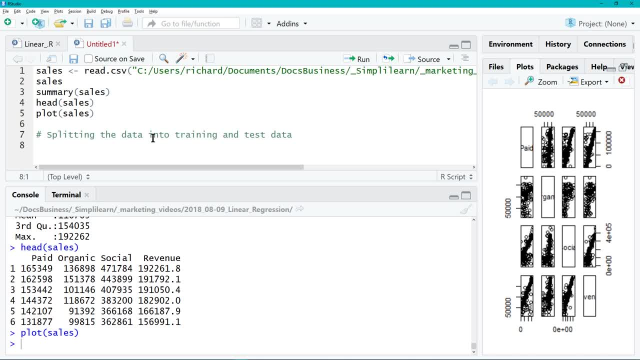 tools. you watch those very closely. You watch your training set and how it does versus your testing set, And if your training set starts doing better than your testing set, then you're starting to over-evaluate your data. So that's a good sign. So that's a good sign. And if you 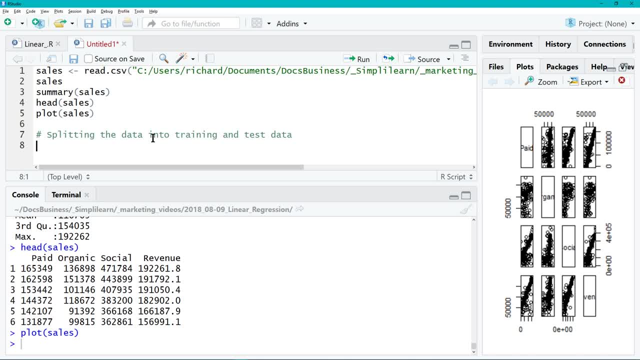 over-train it. Now, that's more with deep learning and some other packages that are beyond what we're working with today. But yeah, this is important. It's very important to understand that that test and that training correlate with each other and gives you an idea of what's. 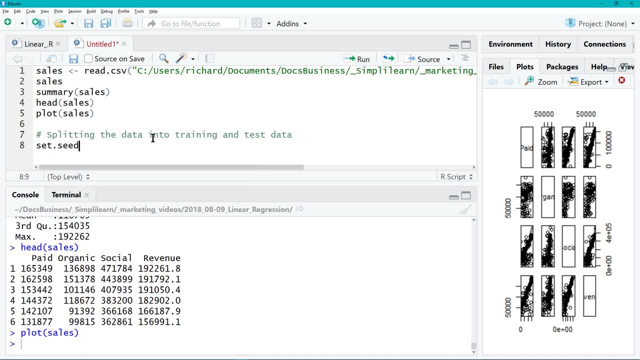 going on and to make sure that you're set up correctly And we'll go ahead and set a seed of two And that's for our random generators, so that when we run them you can seed them with just a random. There's ways to randomize a number or you can do like date and stuff. 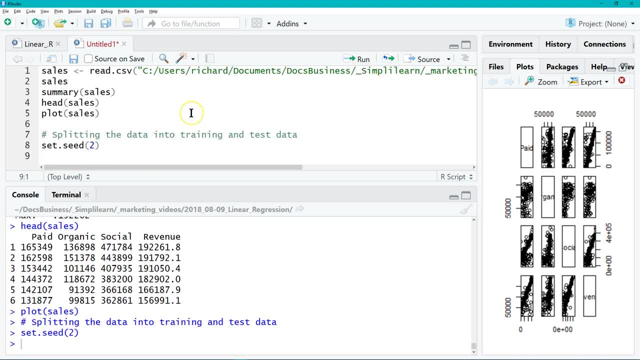 like that, But that way we always use the same random numbers, So we'll seed it with two, And then we're going to need a library. In this case, we're going to import the library And we want to import CA tools And CA tools. 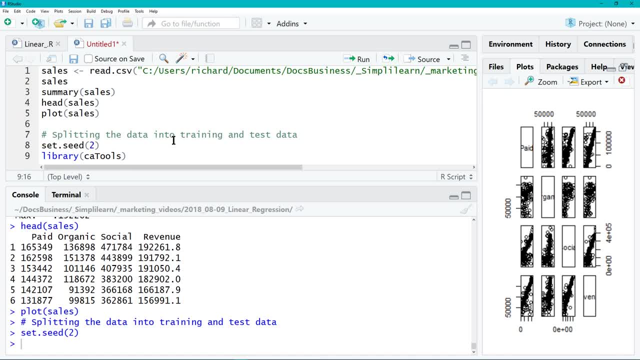 has our split function, So we're going to be able to split our data, along with many other tools we're going to need for this example. So they're all built into the CA tools. That's why we need to import that. A lot of times they call them library, or sometimes you hear 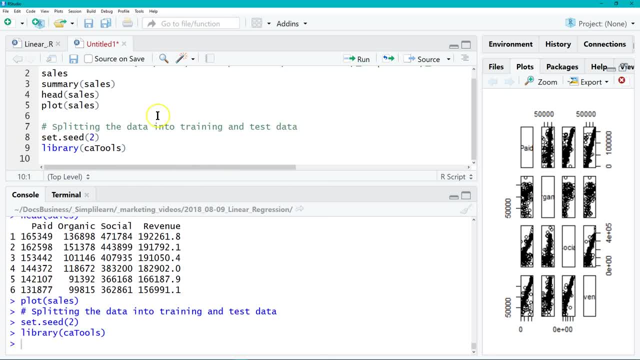 them referred to as packages. So let's go ahead and run that line. And that brings the library in, So now we can use all those different tools that are in there. And then I'm going to do a split And we're going to assign it to the library And then we're going to assign 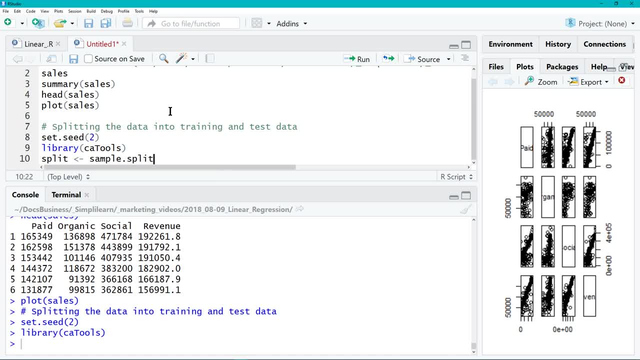 it to the split. That's going to be our variable Sample split. Okay, So that's one of the tools we just brought in is to sample. is the actual keyword or the function word Sample dot split And we're going to take our cells And we're going to go ahead and do a split ratio equals. 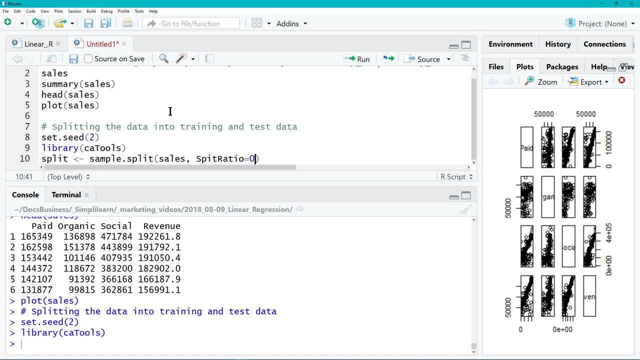 to 0.7.. And let's do 0.7.. So we make sure it knows it's a decimal point or float, And what this is saying is that we're going to take our cells data, the variable we created called cells. It has the data in there And I want to split it. 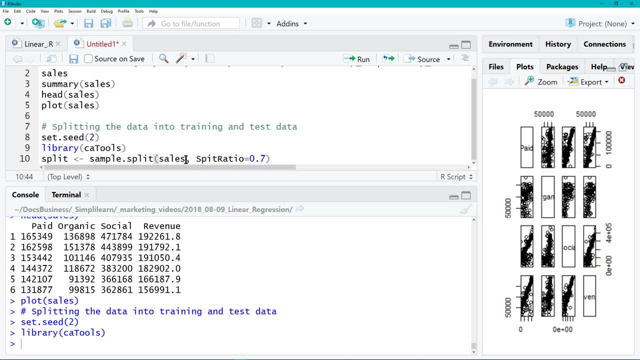 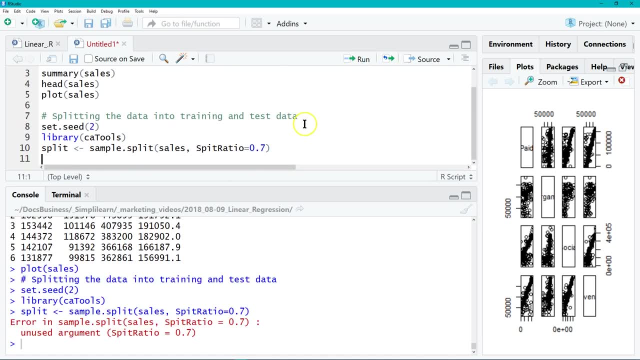 And I'm going to split it so that 70% of it goes in one side- We'll use that for training- And 30% will go into the other side, which we'll use then for testing out our model. Let me go ahead and run that And let's hold on one second. Got an error there. Spit is. 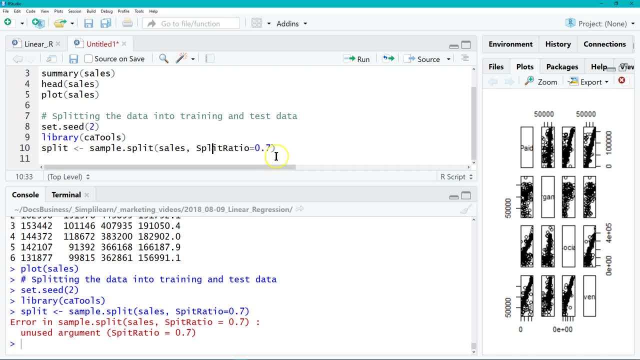 definitely very different than split. I don't think we want to spit our data out- which is actually kind of what we're doing is spitting it out- But we want to split. We want to split the data. Let me get that spelled correctly, And then, when I type in split, we can just: 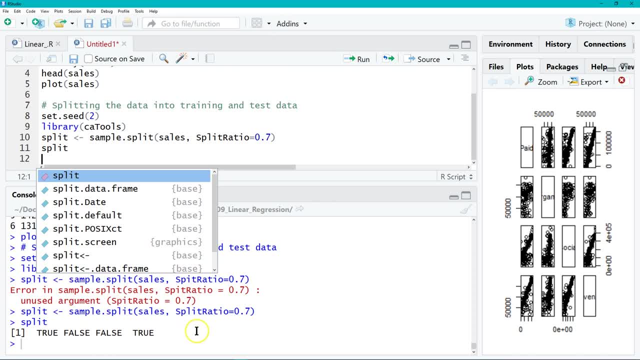 run that because that's now a variable And we can see that it has true, false, false, true. So it generates a number of interesting different statistics going across there, as far as the way it splits the data And right here, if you have not used R in a while or if you're new to R, completely that line one. 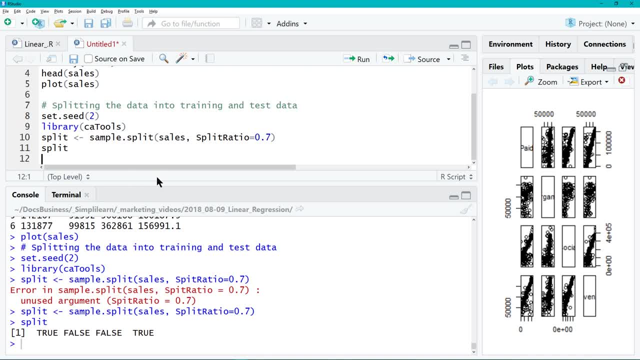 that's what the little one means down there. And then true, false, false, true. That means that's how we're looking at the data. We're splitting all those different pieces of data in line one different directions, And so we now want to create our train set And we're 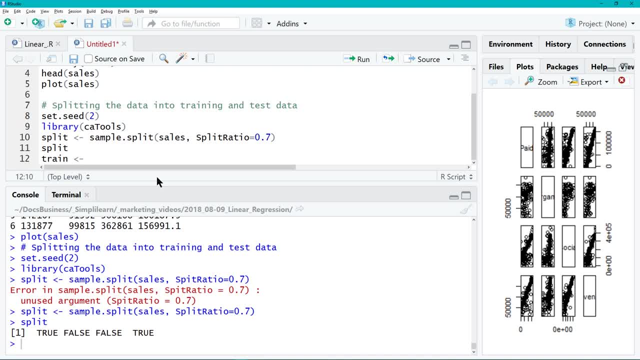 going to assign that And when we take it and we assign to the train set a subset of cells And then the subset of cells is going to be based on split equal. let me put this in brackets, true, So you can see the values down. here is capital T, capital R, capital U, capital E. So I just want. 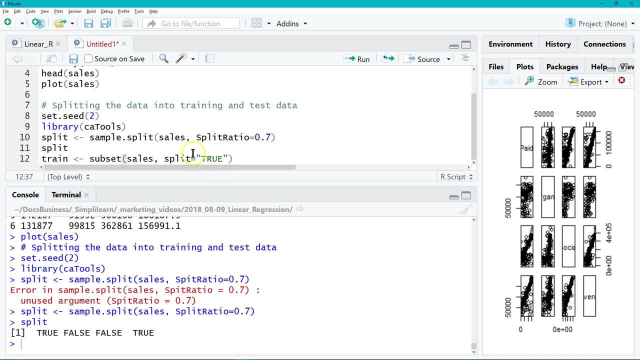 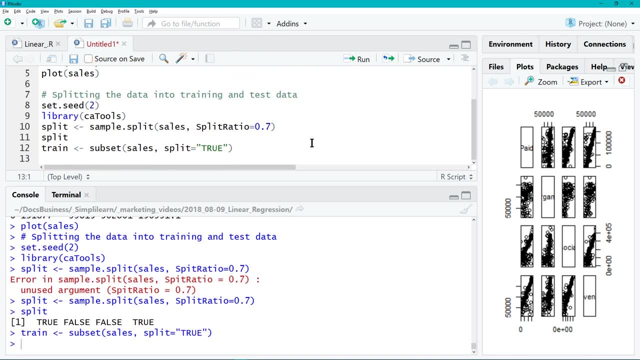 to reflect that on the train And this is going to take everything where our split variable is equal to true And it's going to set cells equal to that And we'll go ahead and run that, set our test variable as a subset of cells and if we assign the true to the train set, then we want. 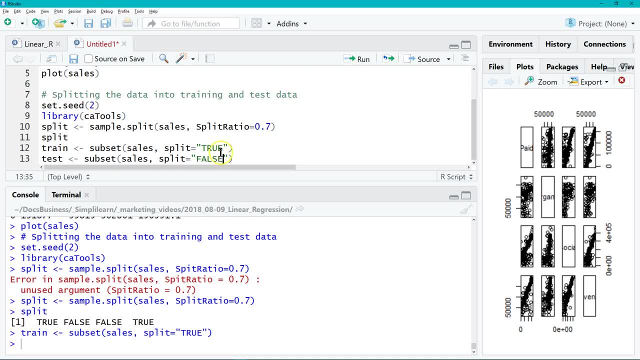 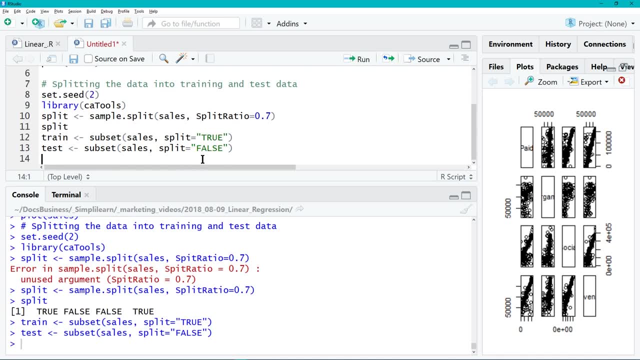 to assign the false to our test set. So now we'll have this will have 30 percent of the variables in it and train will have 70 percent. We'll go ahead and run that. So we've now created both our training set and our test set and we can just real quickly type in train, hit the run on there and you can see. 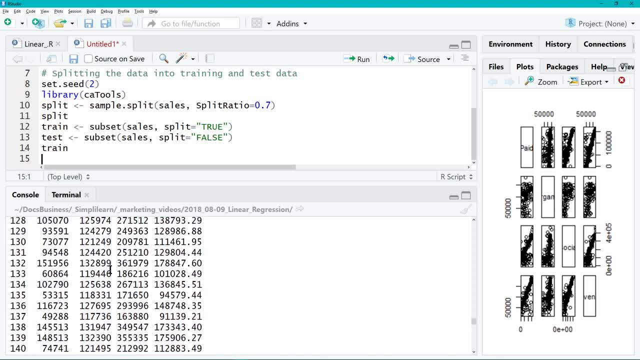 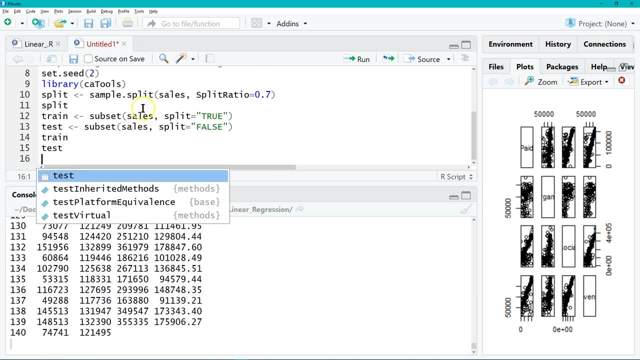 our train set. If I scroll way up to the top, I'll have the column names on there, which should match what we had before- paid- organic, social and revenue- and then we'll type in test. when I hit run on there, that's going to do the same thing. it'll spit out all the test variables going out. So 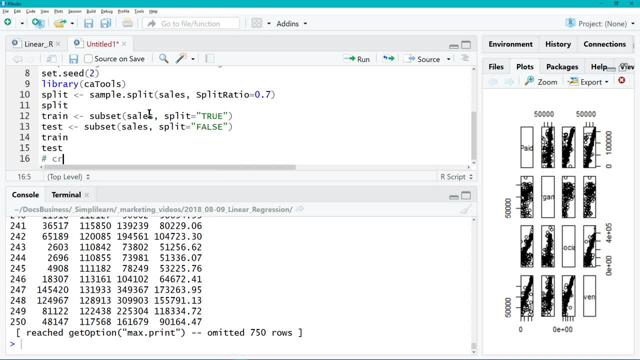 now that we have the test and train variables, we want to go ahead and create the model, and you'll see this in any of the machine learning tutorials. they always refer to them as models. We're modeling a function of some kind on the data to fit the data, and then we're going to put 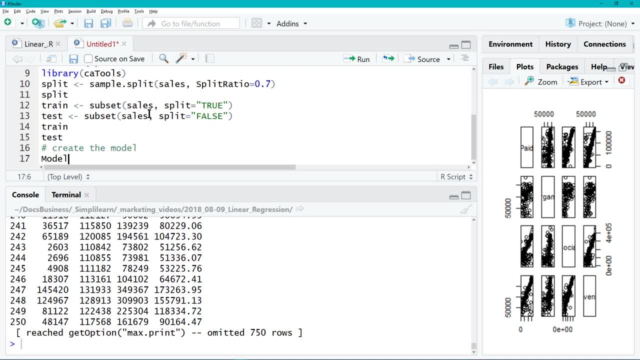 the test data through there to see how well it does, and so we're going to create the variable called models and I'm going to assign that LM. that is our linear regression model. I love how simplified R makes it- just LM- linear regression- and then model M. I guess it dates back as the linear regression. 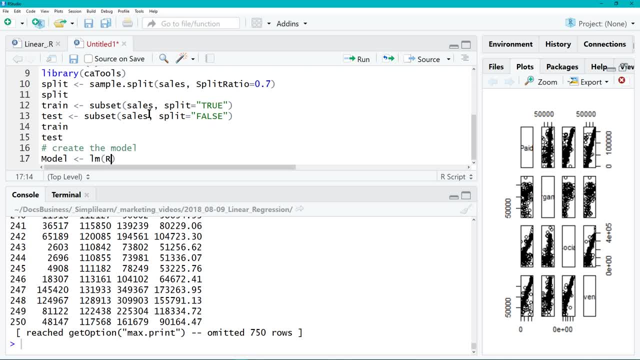 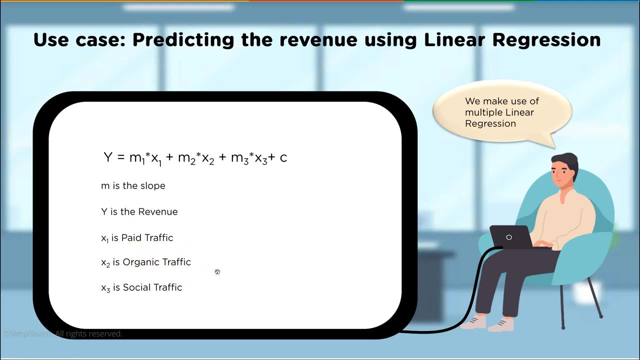 models like one of the first major models used, so they kept it easy on there and revenue happens to be the main variable that we want to track. so, if you remember correctly from our formula, Y is the revenue and then we have X is our paid traffic, X to organic traffic and X 3 our social traffic. so Y is what we 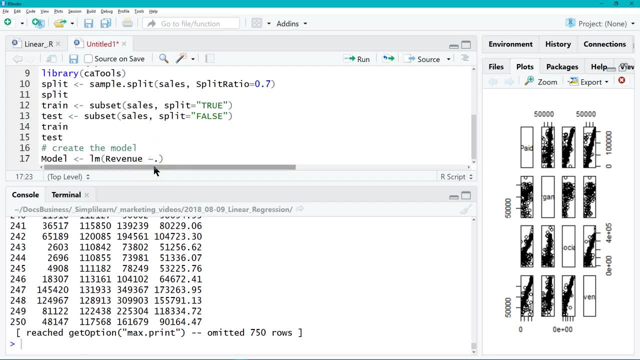 want to predict in here, and then you'll see this notation where we have our squiggle and the period, which means we're going to match up the revenue lines with the lines of the data we're putting in here, and then I'll put comma and then our data equals train and of course that's the training data that we 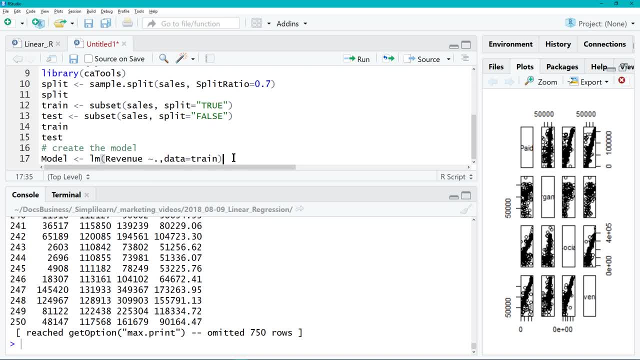 created. so when I hit the run, remember we did all that discussion about all those different functions and formulas to compute our model and how that set up. when it comes down to it, we spend all our time setting up our data and then I hit the run button on the single line and our models been trained. so we now. 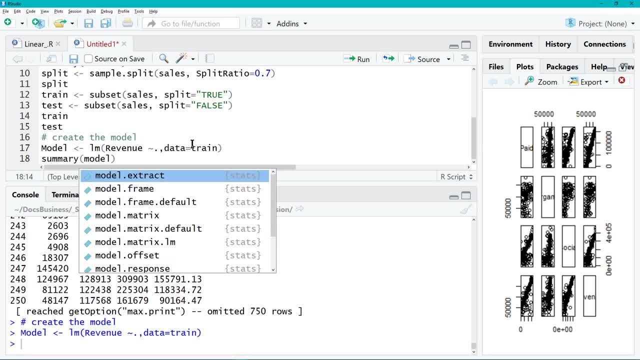 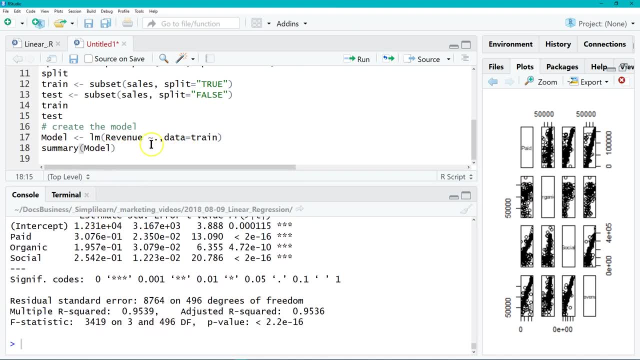 have a trained model here and we can do a summary of the model. summary is such a wonderful command because you can do that on our. that works on all kinds of different things on there. oops, and of course it does help if I remember that my model has a capital N when I run it and you'll see right here tells you a. 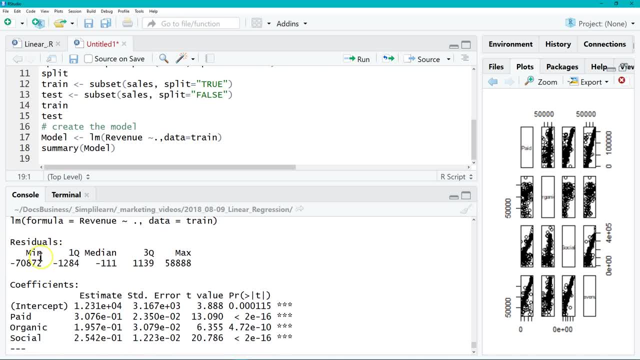 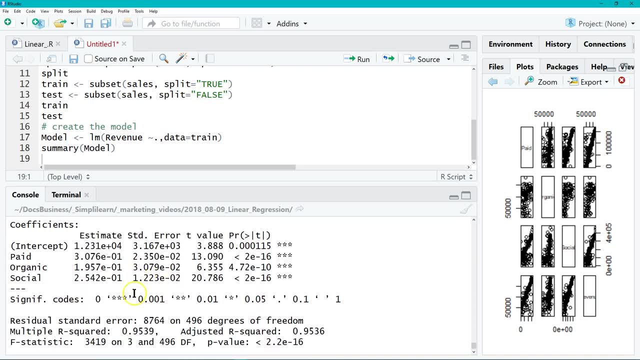 little bit about the model use. a summary on there comes down here. it has our residuals. this is all the information on there. as far as, like, the minimum, the median, the max has all our coefficients in there, if you remember correctly from our formula. let's just go ahead and switch back over to that. we have m1- x1. 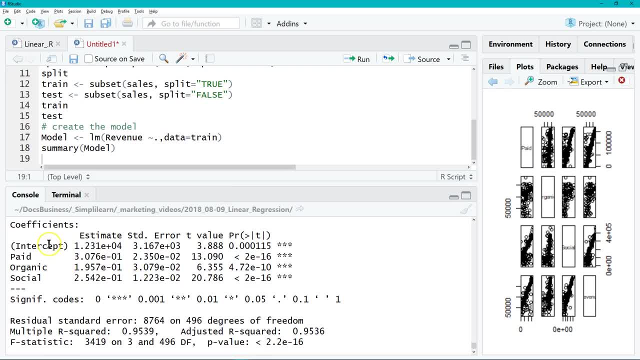 m2, x2, m3, x3 plus C. well, that's right here. here's our intercept, and then we have our different values for each of these. so you have our intercept, our paid, organic and social, and then it also shows us error and information on the. 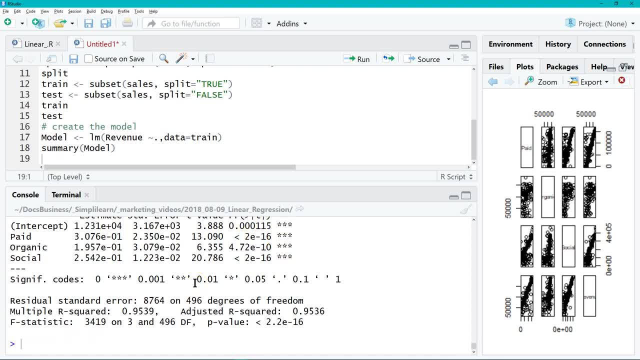 error and one of the really nice things about when you're working with our. you can come down here and you can see that we have our values and we have our data, and then you can see that we have our data in here and you see where we. 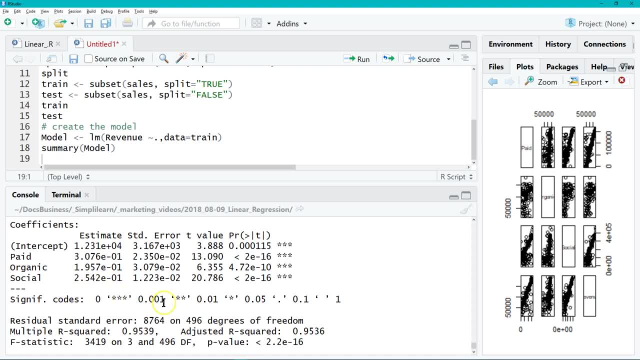 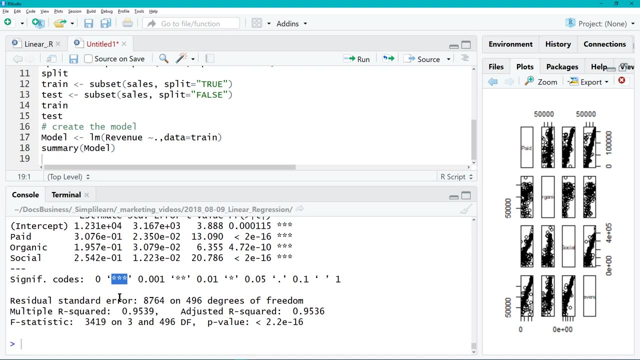 have our stars down here and it says three stars, really good, two stars, maybe one star, probably no correlation. and we can see with all of these it has three stars on them. so out of three stars we get three stars, and all these there's no four stars. four stars would mean that you have the exact same data going in as 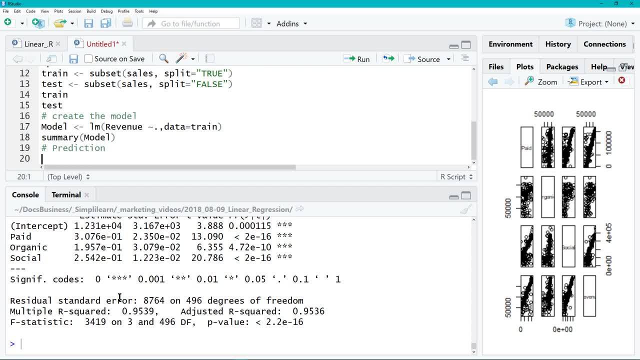 coming out and then, if we're gonna do this, we want to actually run a prediction on here, and that's what we saved our test data for. so let's come our prediction. we'll take this variable and we'll assign it predict model. remember, the predict comes. 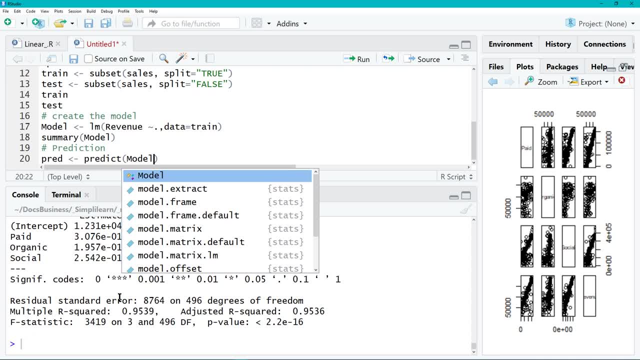 from when we imported that package, the ca tools. that's all part of the ca tools in there. so we're going to predict, we're going to use the model and then we're going to use our test data. pretty straightforward, quick and easy. we'll run this and then, if we go ahead and type in the predict, 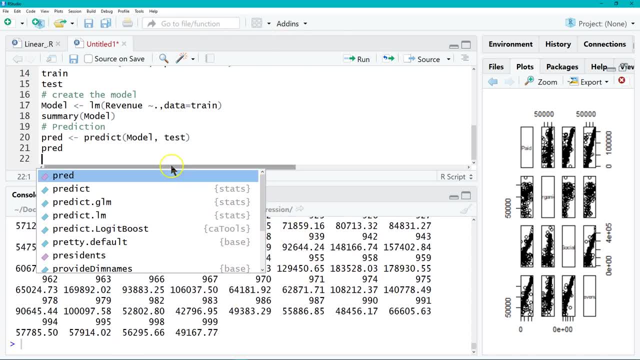 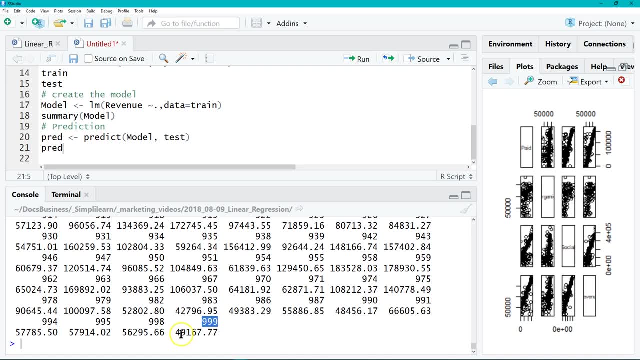 it'll print out what's in that variable and you'll see down here the predicted values it expects to come out. it's going to see our revenue is and it goes through and it gives it both the line number and the actual revenue value. so that's quick and easy, boy. we got a prediction really fast and this: 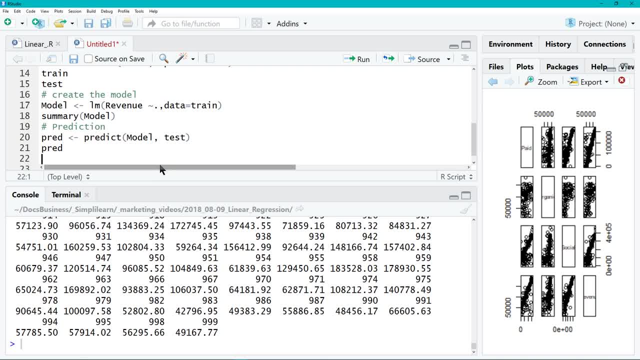 is also how you would do it if you had new data coming in after this. you could predict the revenue based on these other factors. so, now that we have a training model which or we train the data with our training data, or we trained the model with our training data and we've done a prediction on our 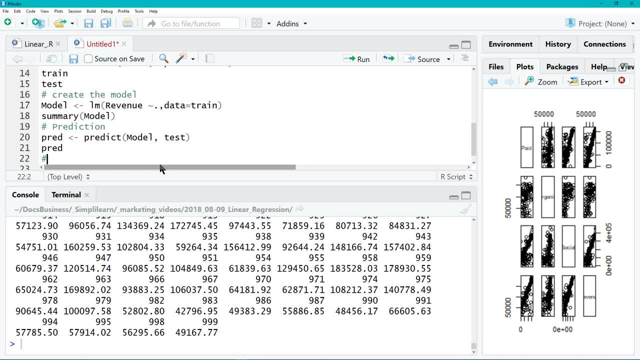 model with our test data. we want to look this up and we took a quick glance from our training thing. our training said it trained really well, but that's not the final word on it. the final word is going to be comparing it. so we want to go ahead and do comparing- predicted. 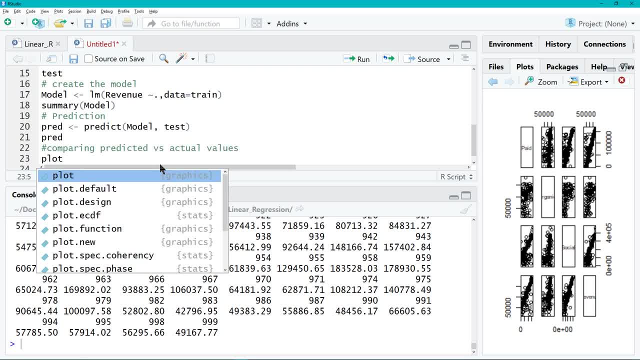 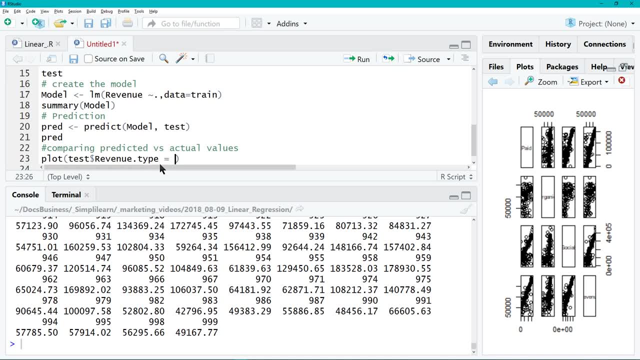 versus actual values. what I'm going to do is I can do a plot and I can do our test and we're going to do test revenue: dot type equals. we can put this in as a type type 1 and or L, and then we have LT y equals one point eight and we're going to set up for column blue. 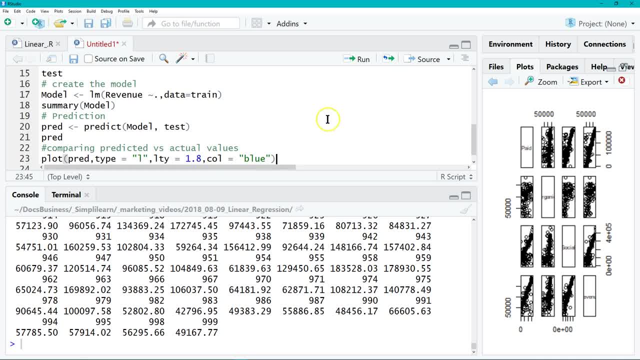 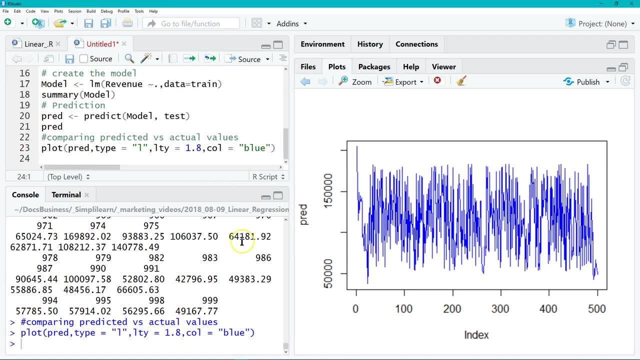 that's a lot of stuff in there. let's go ahead and just run that so you can see what that looks like and what's that stewing. it's going to generate this nice graph. we see on the right. there's our graph. you can see the data comes up and down. be plotting the prediction on there. so this is the. 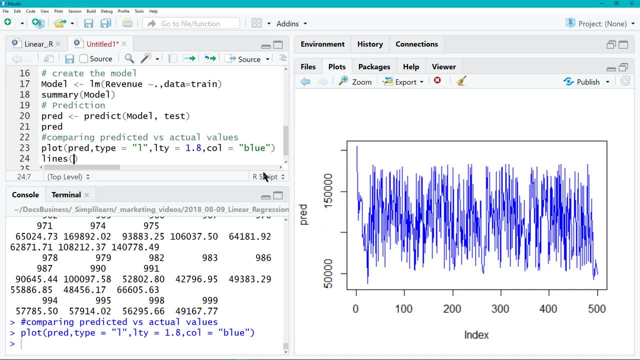 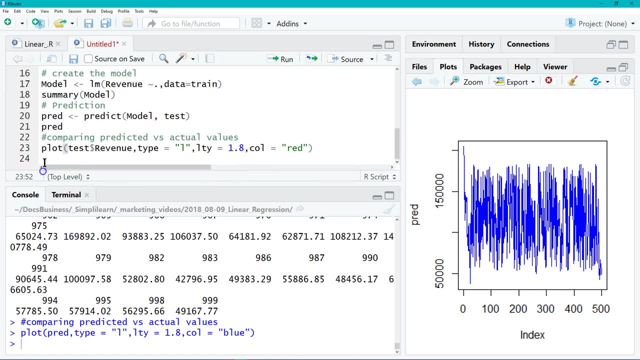 values we predicted, and then let's go ahead and do lines- and I actually did this backwards, so let me try that again- and we'll start with the red one. we're gonna do the first one in red and I want to start with the actual test revenue. so here's our test revenue and we'll go ahead and run this. 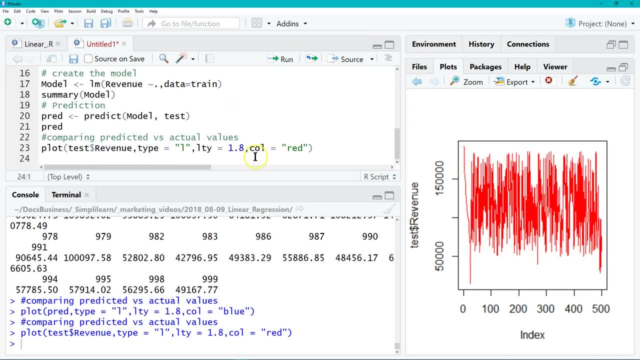 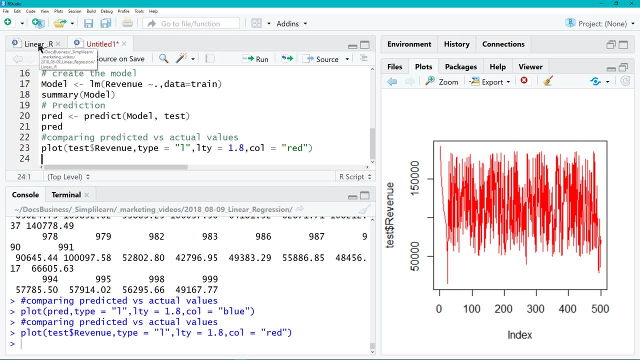 and so we have our red plot over here in red. go ahead and take a look at that and pull that over. you can see how that looks. goes up and down, hard to track there. and then we're gonna do a couple things here. we'll plot our test revenue and then we'll make it a little pretty of those kind of. 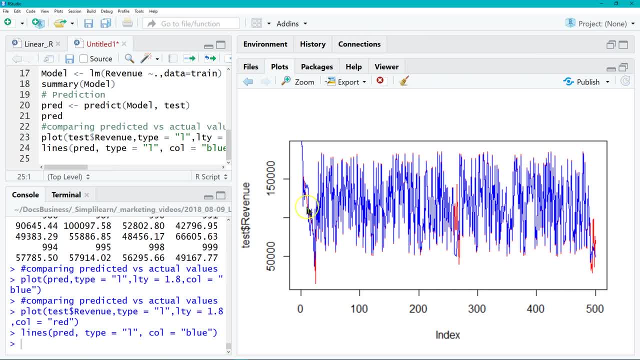 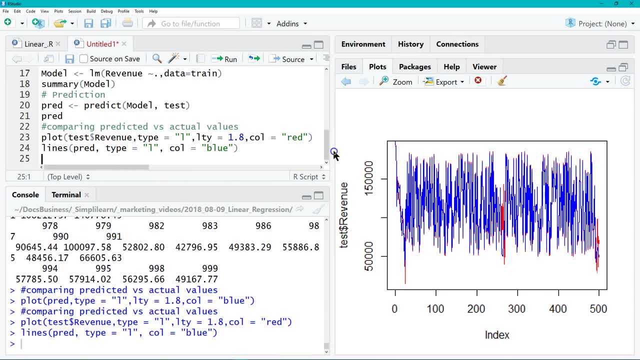 hard to say. see the way I was crunched up here on the right as far as size and sizing and everything. but we'll go ahead and have our columns in blue and run our prediction on there too. you can see they overlap the two graphs. so we have our test revenue and then we're going to run our test revenue. 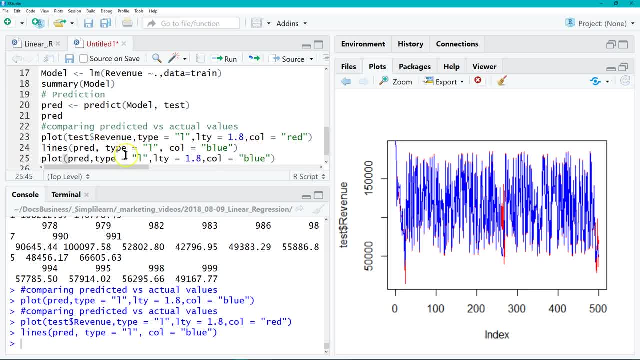 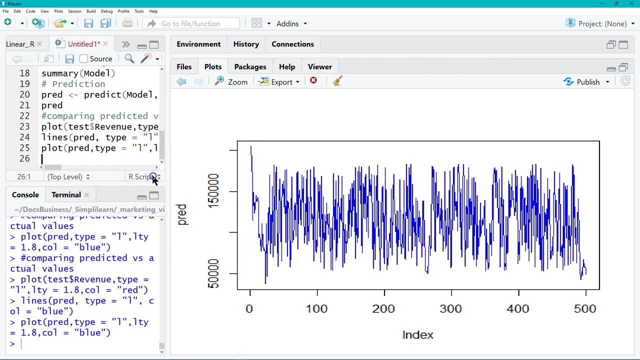 and our prediction. and then, finally, what I started with is we'll go ahead and plot the prediction fully on the bottom and run that and if you look over here on the graph, we put the blue lines over the red lines and so you'll see a couple spots where there's red underneath there. but for the 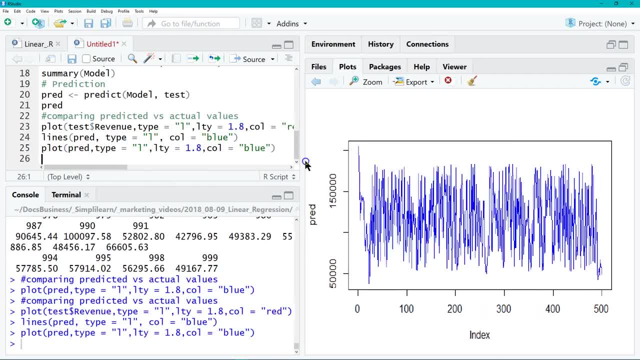 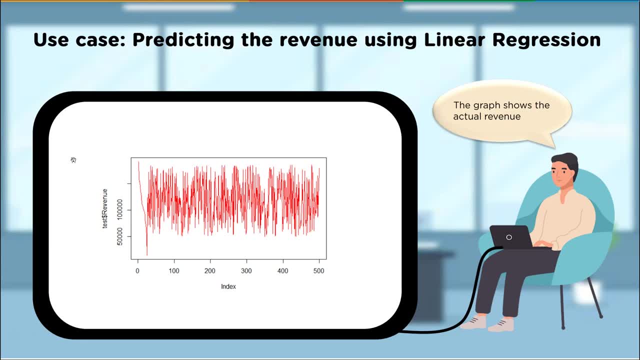 most part our predictions pretty right on, so it looks really tight, looks like a good set of predictions for what we're working on and this is what we were looking at the slide right before we started diving into the RStudio. we can see in the slide here: here's a red. this is a little bit. 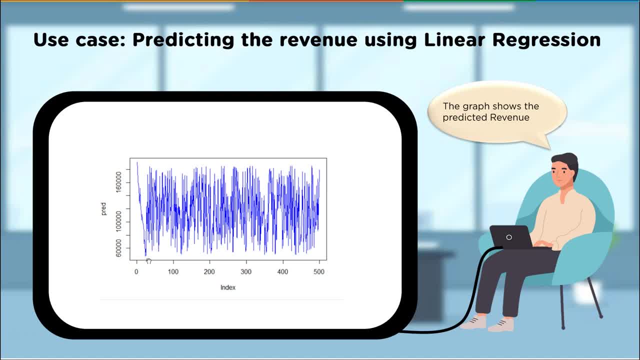 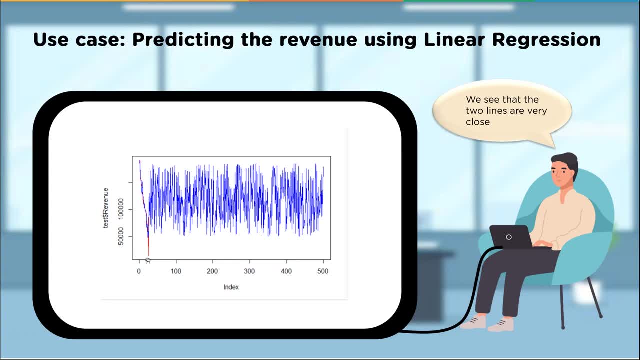 better spread out than what I have on my screen from my RStudio. so we're going to go ahead and run our RStudio and the graph shows a predicted revenue. we see that the two lines are very close so again, they're tight. it's right on. this is what we're looking for in our prediction model, but it's 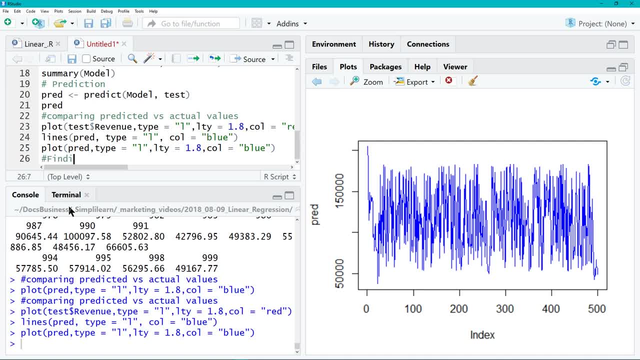 not good enough just having a graph, and you always do both. and the reason we do both is you want to have a visual of it, because sometimes you look at these, you get to the graph, you're like, oh my gosh, what is that? and then sometimes you look at the graphic- oh, that's right on. how come my accuracy? 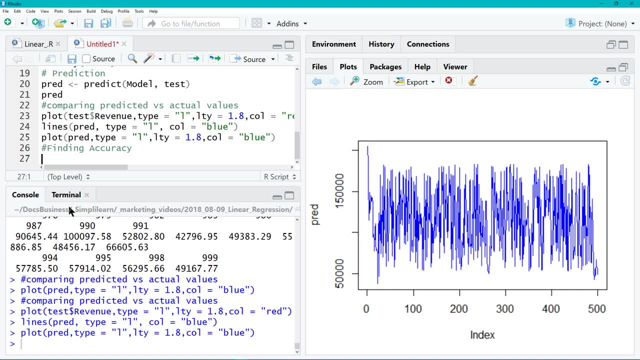 doesn't look right and you realize that your accuracy might be off or you're plotting it incorrectly. so let's go ahead and look at the graph and we'll look at the graph and we'll use the variable name we're going to give it and sqrt the square root of the mean, and mean just means average. and then we want prediction minus. 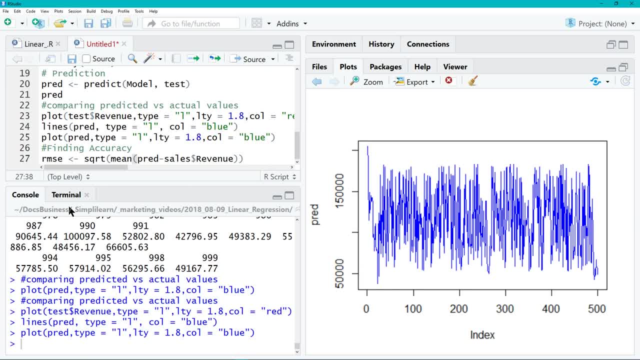 cells revenue, and then we're going to take this whole thing and we're going to square it. so what we've got here is we're going to go through. let's just explain this formula we're using is I'm going to look at the, what I predict it for to be and what the actual cells. what's our prediction versus our? 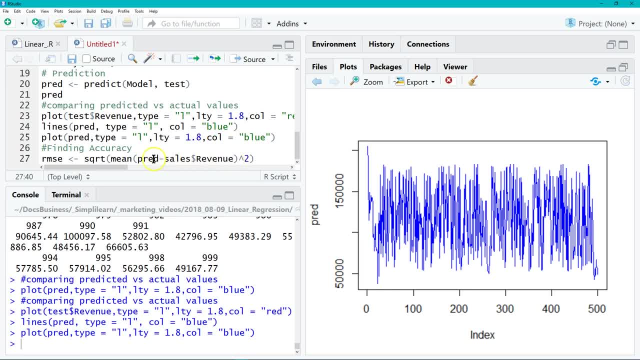 cells and what's the actual sales. so what's our prediction versus our sales? so what's our prediction versus our sales, comparison to the revenue? and we compare those two, we're going to find the average and then I'm going, or we're going to square each one of those values and then we're going to average. 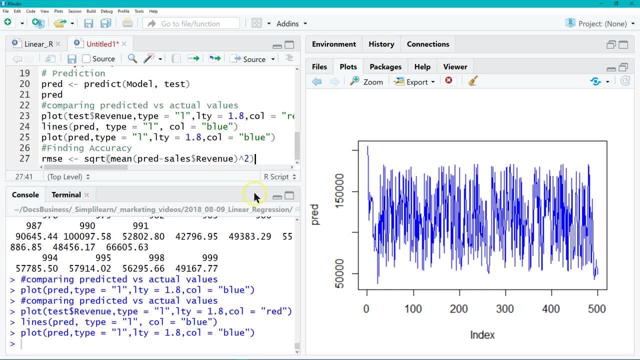 the square and then find the square root of that, and that's quite a mouthful. the reason we do it this way, the reason we square the value and then we find the means- is to generate an answer based on- doesn't matter whether it's plus or minus. there's a lot of other formulas you can use there. 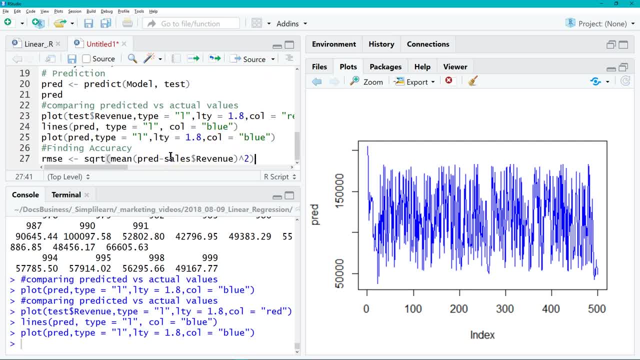 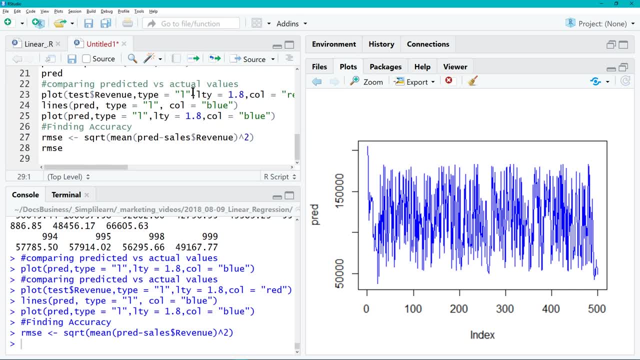 to check your accuracy and all kinds of other things you can do. but a quick, straightforward way of doing is just like this: and then let's go ahead and run this and then we type in the RMSE and they'll give us an actual printed value out. let's just see what that looks like. and so we have. 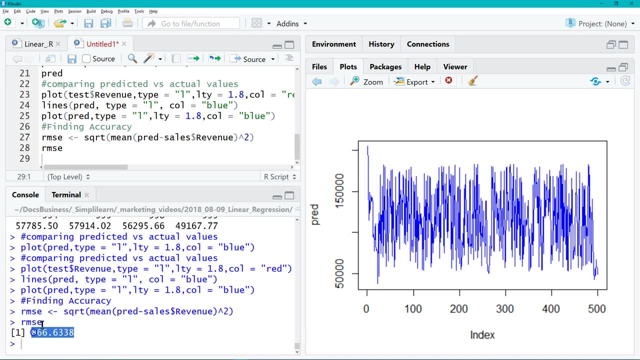 eight, sixty six point six, three, three, eight for our accuracy. and so we look at the eight hundred and sixty six point six, three and we compare that to say fifty thousand. that's pretty close, that's. that's actually a pretty good accuracy, given this model takes a little bit more when 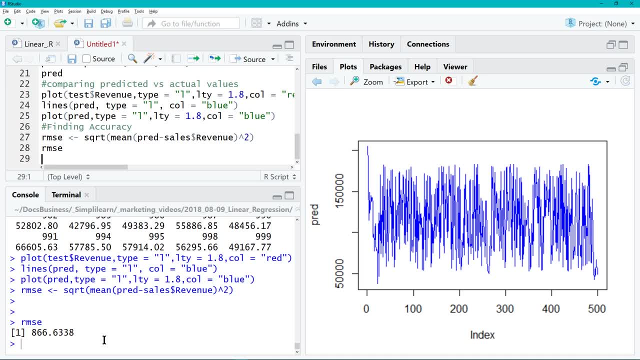 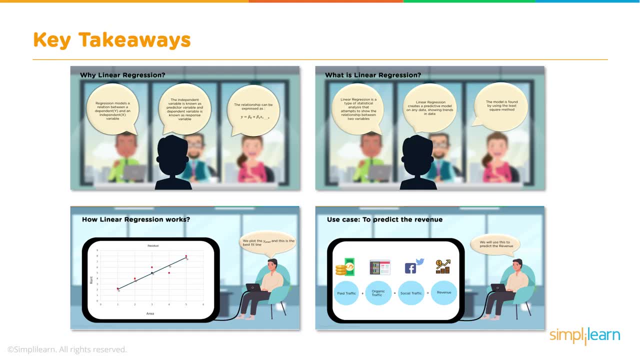 you're playing with accuracies and start dividing out other different aspects of it to get something you can communicate better with, but you always start with the square root means that's always a good place to start. so what are the key takeaways for this? why linear? 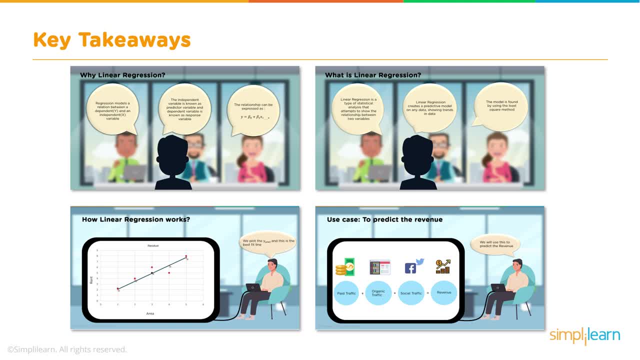 regression. regression models a relationship between dependency Y and an independent X variable. the independent variable is known as a predictor variable and the dependent variable is known as the response variable. the relationship can be expressed as: Y equals beta naught plus beta 1 X 1 plus beta 2 X 2, etc. and we looked at what linear regression is. and we looked at what linear regression. 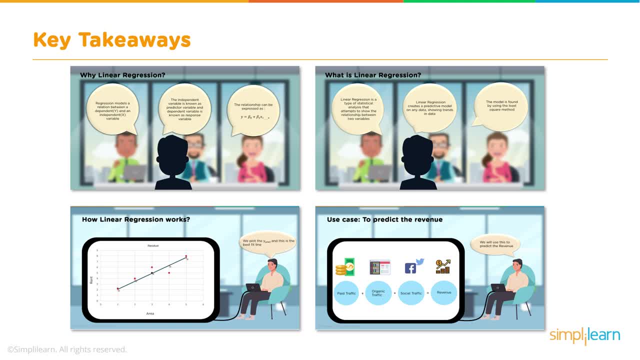 is. linear regression is a type of statistical analysis that attempts to show the relationship between two variables. linear regression creates a productive model on any data showing trends in data. the model is found by using the least square method, and then we looked at how linear regression works. we plot the Y, predict and this is the best fit line, whatever is going to have. 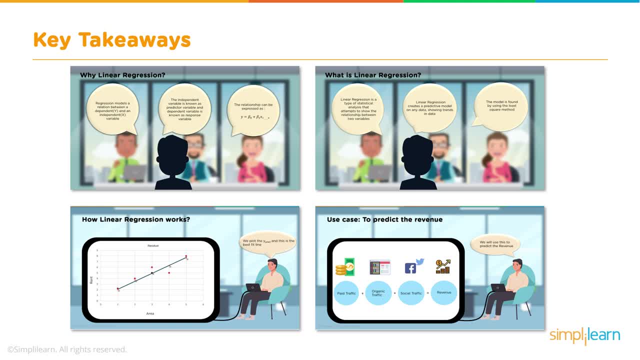 the minimal error on it and use case to predict the revenue. we looked at being able to generate a model that allows you to predict a revenue. now, a lot of times when you're studying machine learning and you get into deep learning or any of the other models, almost all of them have some math based on. 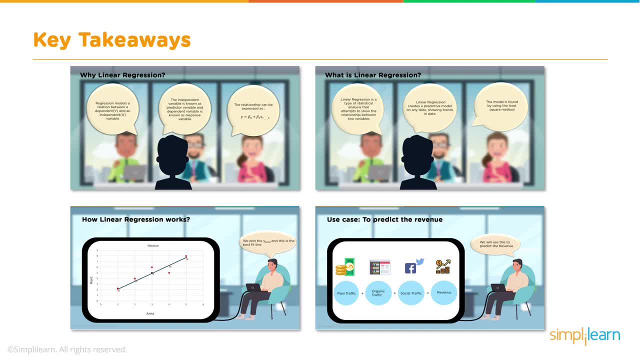 this linear regression model. this is the basis of so much and if you're starting with any new data, this is a good place to start because it helps build a very solid function you can look at and usually can predict a lot of things, or you can take this prediction and put it into your next. 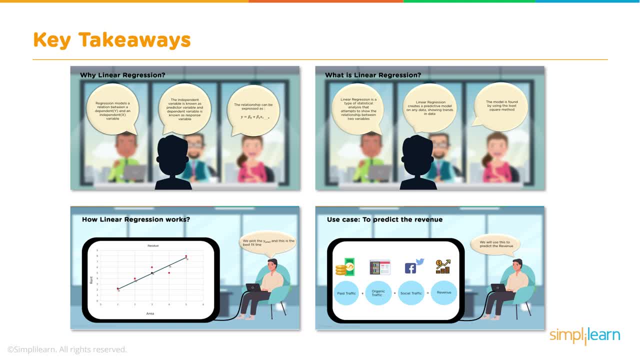 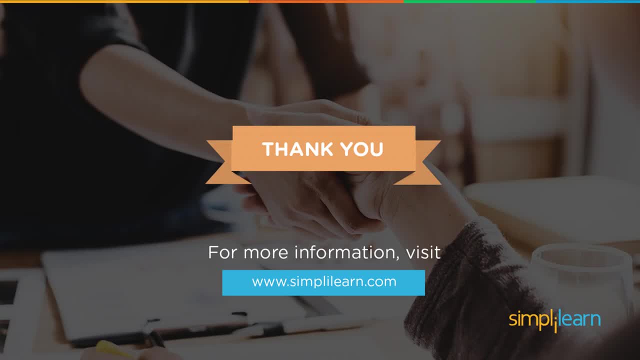 step, which would be to look for outliers, things that don't match the linear regression model, and find out why, and find out other information about those areas so you can better predict them, in which case we'll wrap up our linear regression model in R today. thank you for joining us for more. 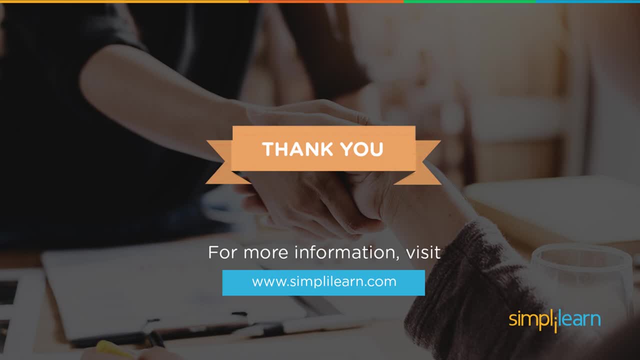 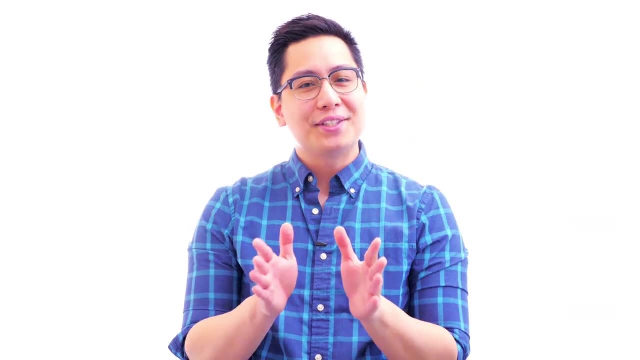 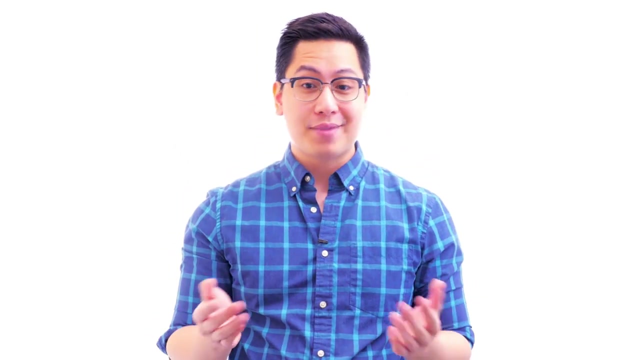 information: visit wwwsimplylearncom. get certified- get ahead- hi there. if you like this video, subscribe to the simply learn YouTube channel and click here to watch similar videos. to nerd up and get certified: click here.